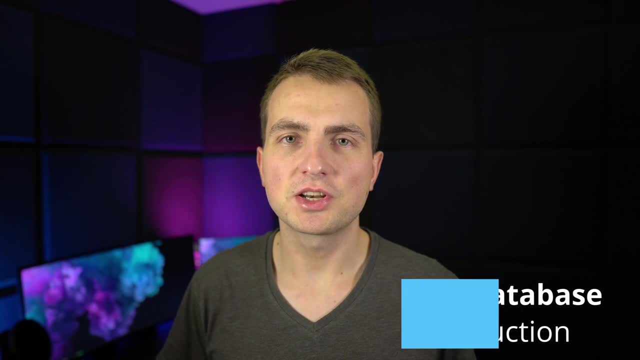 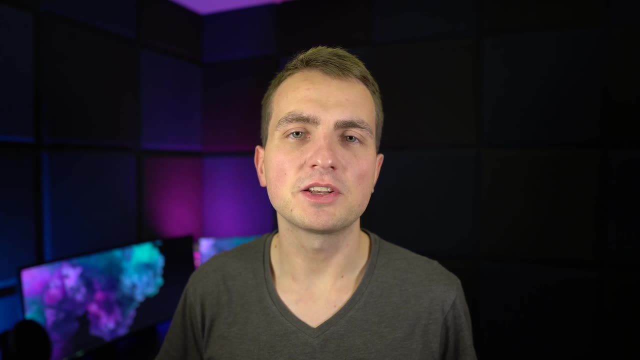 Hello everyone, this is Adam and I'm back with another interesting topic. Today we're talking about SQL database. If you need to manage, query and ensure structure of your data in database, this is one of the primary services to do so. So let's jump straight to it, shall we? 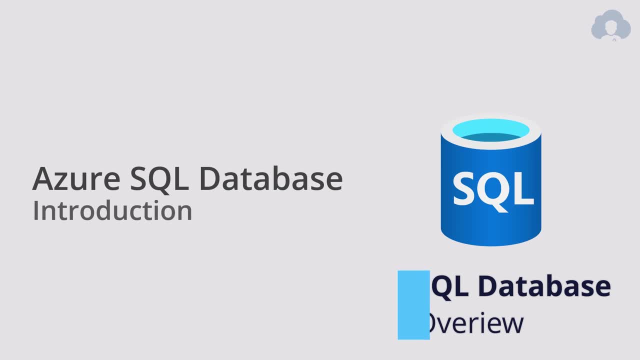 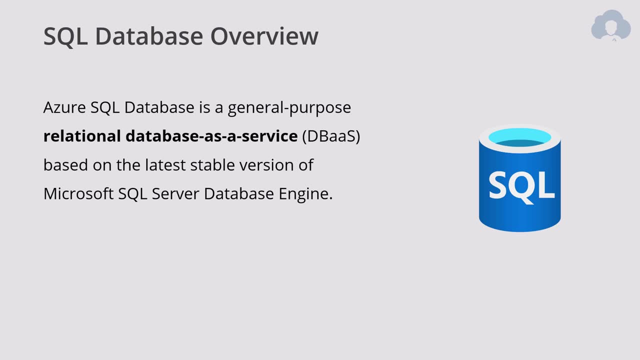 So to talk about SQL database, we need to understand the basics. So SQL database in Azure is a relational database as a service. That means it's a latest stable version of Microsoft SQL Server Database Engine in the cloud. But let's get down a bit more to basics. What is relational database and why would you want to? 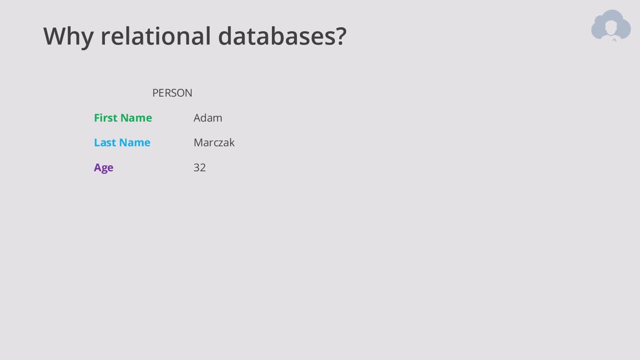 use it So, in case you have an entity called person and this entity has three values- first name, last name and an age- you can actually start putting those values as columns- So first name, last name and age- and create a table. so within this table you just input your values into appropriate. 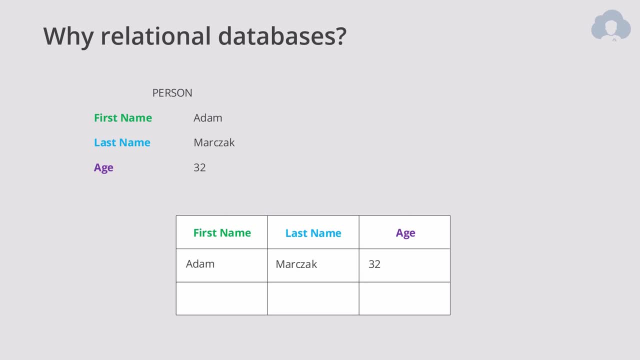 columns. that's fairly simple, right of course, when another entity comes, for instance John Mayer, you just input this as additional row. but relational databases are a bit more than just table and rows. it's all about defining a table- in this case person's table- but also defining something called constraints. so 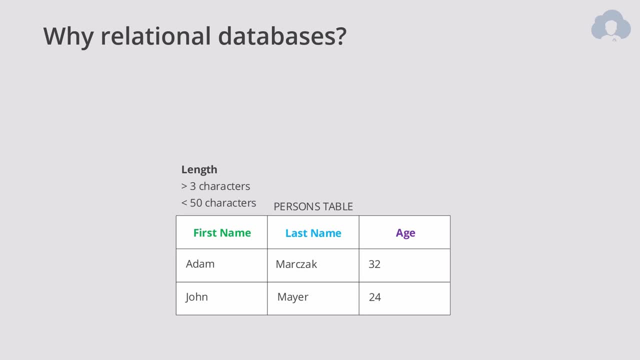 you can say that your first name it must be longer than three characters and shorter than 50. and for age you can say that must be of type integer, to make sure that only integer values are there. but also you can say that the value must be lower than 130, so you can define those constraint to ensure that data. 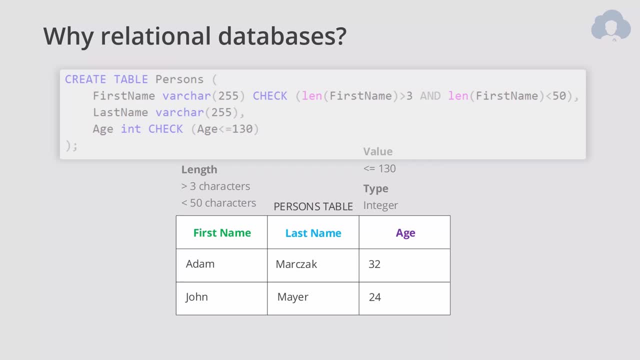 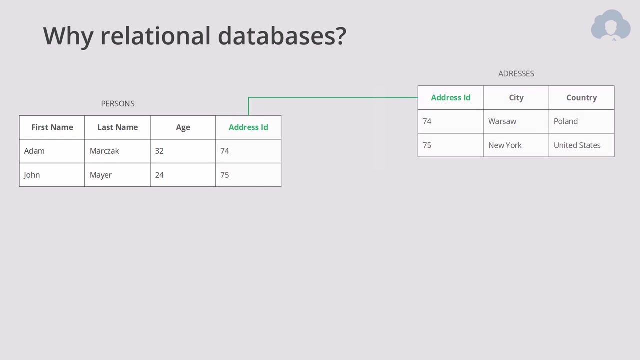 quality is there and you can also do that with a simple SQL statement, creating table and all those constraints in a very simple manner. but that's not where it ends with relational databases. you can actually use multiple tables. you can actually use multiple tables. so if you have a person table, you can define addresses table and combine it. 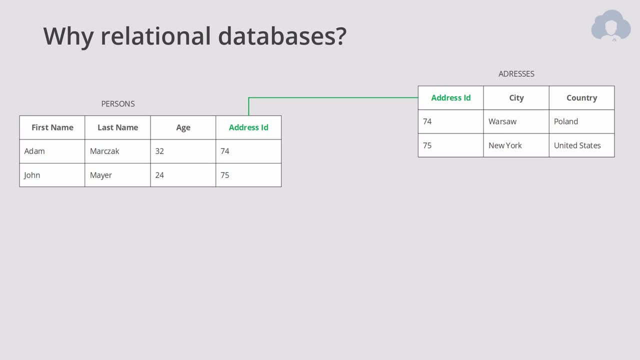 using, for instance, address ID, and it's up to database to ensure that, based on the relational definition, it's making sure that the rows are matching from all the tables and it's up to you define what kind of relationship you want between your tables. of course, if you want, you can combine multiple tables. 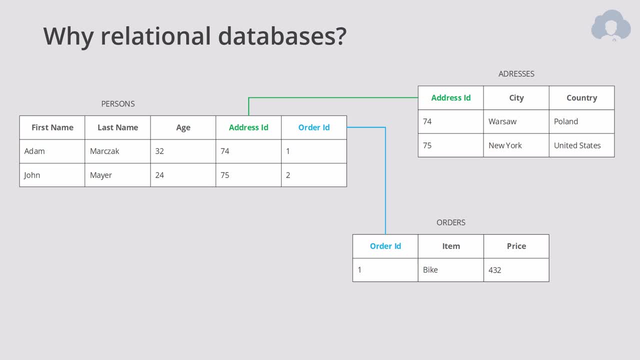 using relational database models and of course, once you do that database again, the quality stays there. but what is great here is that if you have all those relationship defined you can actually combine data from multiple tables using SQL queries to, for instance, calculate how many orders where there per country. 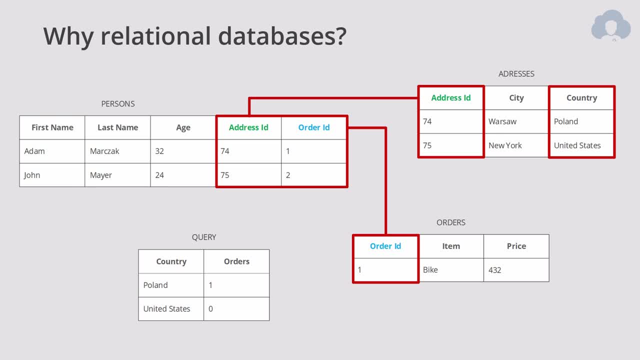 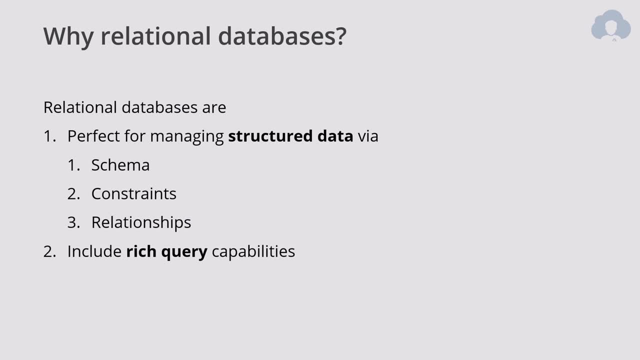 this is a powerful feature of the relational databases. so why would you use? use relational databases? well, for, of course, because if you're using structured data, you can actually manage it very well using schema constraint and relationships in general, and you can use the schema constraint in your database to actually manage your database orders using SQL queries. 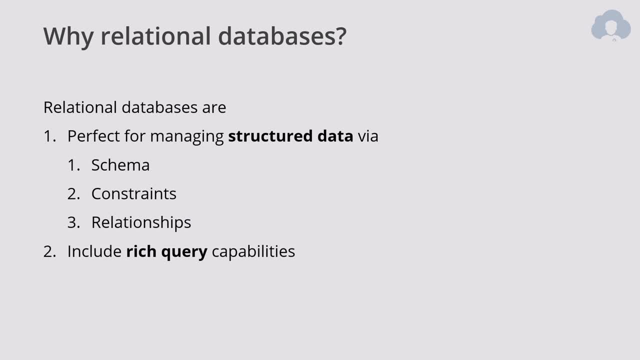 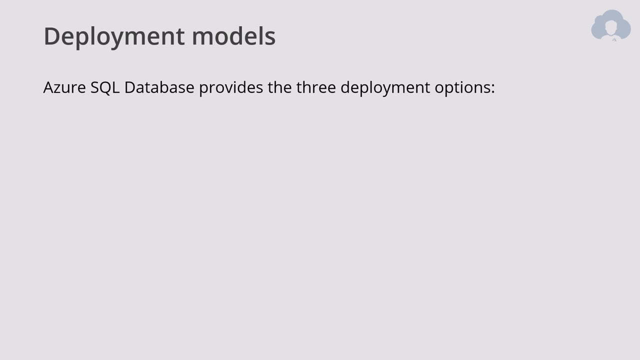 but also if you want to use those rich wary capabilities to explore your data, then relational databases are perfect choice for you. with that said, we can actually go to the database itself, the Azure SQL database. Azure SQL offers free deployment methods. first, one is a single database. it's a fully isolated 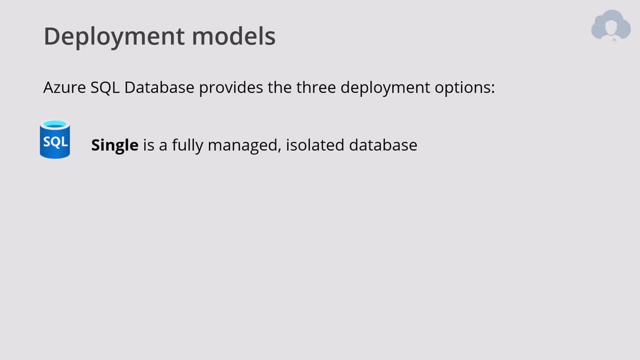 and fully managed database for you. so, simply said, this is a SQL Server migrated to the cloud and redesigned a bit to fit the cloud needs and clouds capabilities. you additionally have something called elastic pool, so you can actually have multiple single databases that would share resources across there. 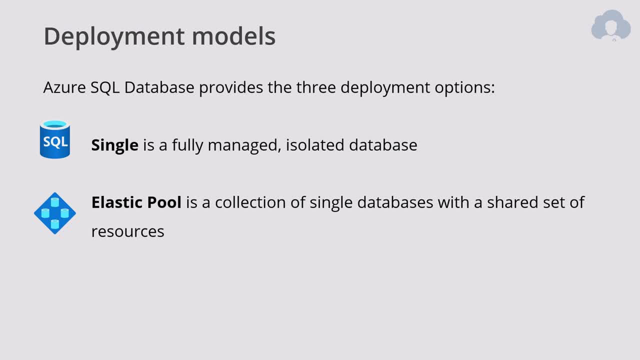 are several scenarios where we usually want it and we're gonna talk about those in couple of minutes. and the third option is manage instance. so, since single database is migrated SQL Server to the cloud, why would you want to use SQL Server as a single database and why would you want? 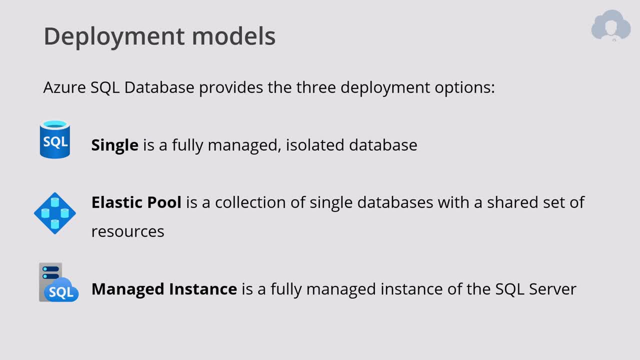 managed instance because single database, when moved to the cloud, had to get rid of some features in order to be really cloud ready solution. but if you need a full capabilities of this SQL Server and you want to manage all those capabilities by yourself, manage instance is there for you. of course, it's the most. 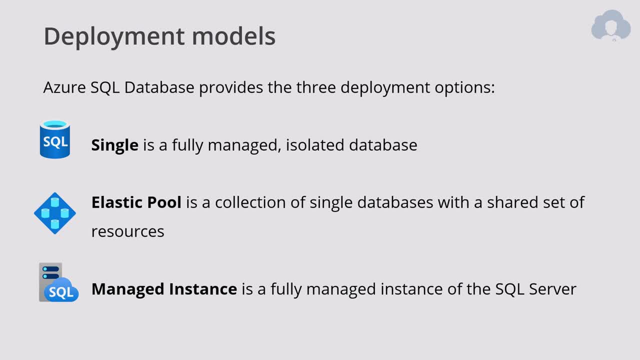 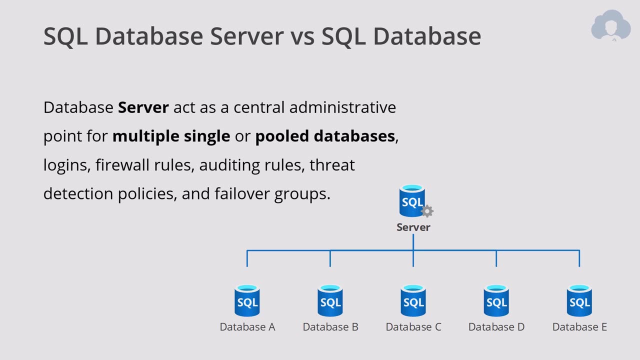 pricey of all the options. so make sure that you only use it for lift of shift scenarios or where the set of features that you need are only available on the SQL Server on-premise. otherwise, always try to design for a single database in a cloud. so one important thing to understand here is when you're gonna be creating. 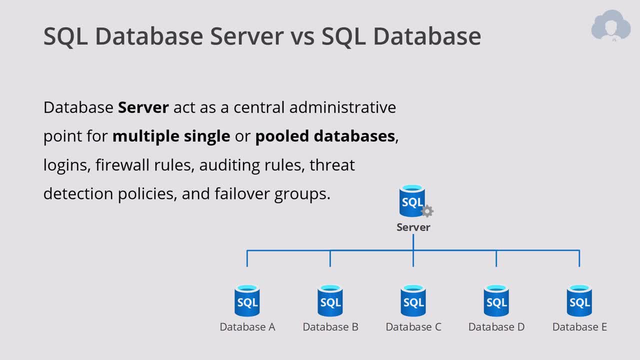 SQL database in a cloud. you're gonna be actually creating two objects. one of them is SQL Server database and the second one is SQL database server. so the server. think of it like a logical unit. it's a central administrative unit where you can manage your single database or pooled database, what kind of things like logins. 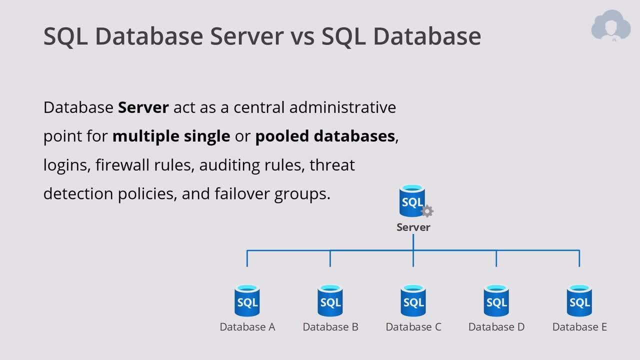 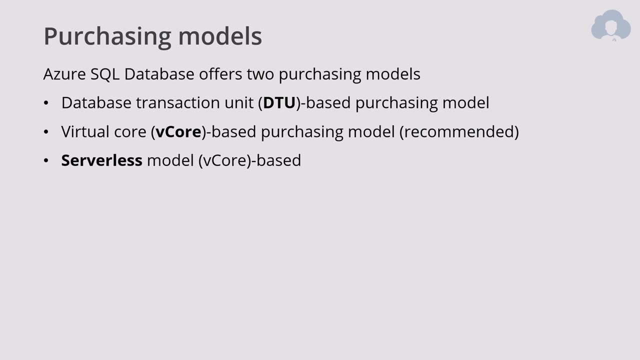 firewall rules, auditing, threat detection, etc. etc. and a single server can contain multiple databases. if you've been working with a skill server on-premise, this is pretty much identical here and Azure SQL database offer you to buy database in free, pricing tiers- or maybe not pricing tiers- by pricing models. 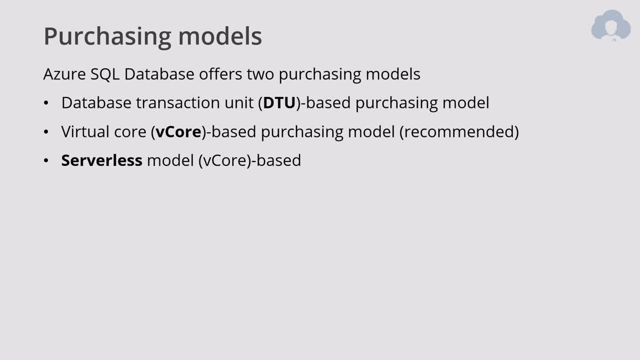 first one is DTU. this is the database transaction unit. it's Microsoft unit of performance, something like in the middle between vCores, memory, IOPS and other metrics. but it's really hard to estimate this way and recently Microsoft introduced a vCore base, so you basically buy virtual course. this is a currently 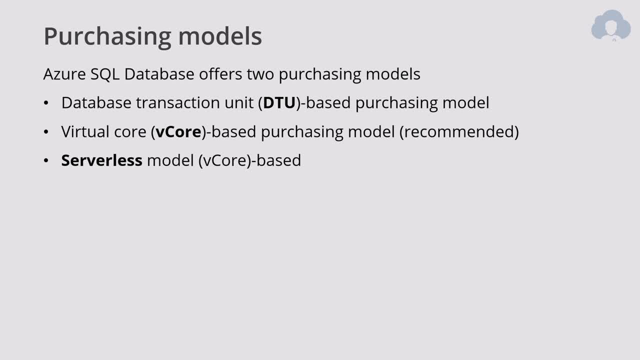 recommended way to buy it and it's also easier to estimate if you're moving from on-premises. you most likely already know how many virtual cores do you need for your database to be really well suited for this. and lastly, you have serverless, can't? it is a vCore and I will talk. 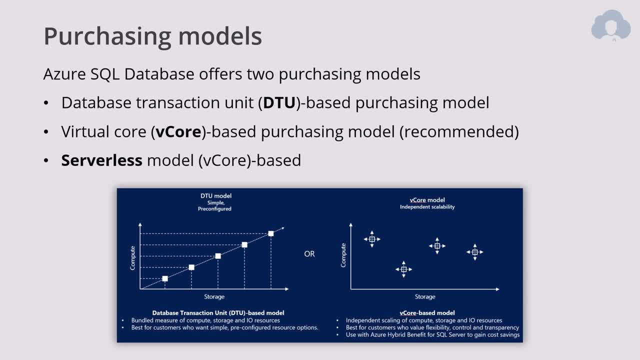 about serverless just a bit. the major difference here is that for DTU you scale storage together with compute so that twice the compute the twice the storage you get, which is not ideal because even if you're not using that storage, you get twice the storage with every. 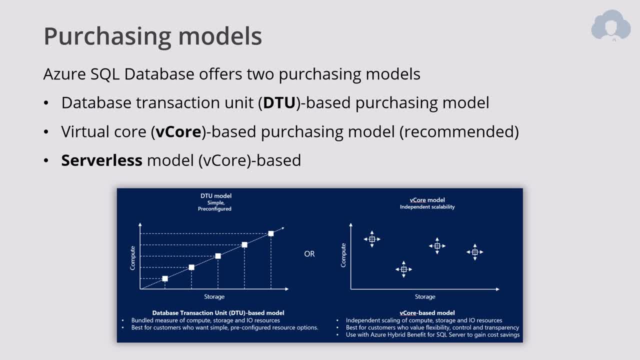 thing to your app. but with vCore you can actually scale storage independently from the compute. so you can say: I want only 5 gigs of RAM and 5 cores and then 100 of gigs of memory- sorry storage. or other way around you can say: I want very. 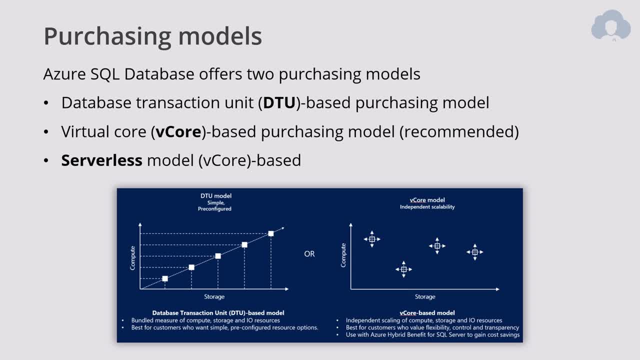 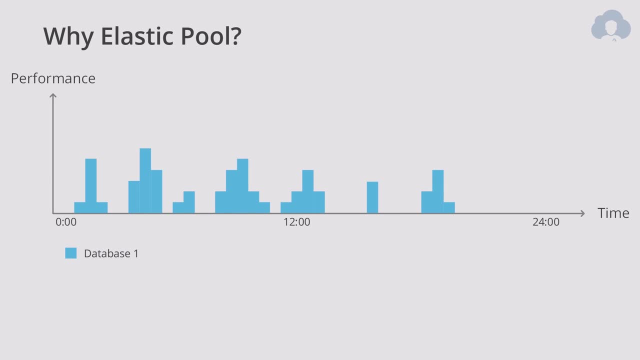 small storage, but I want very powerful machine. additionally, because this is a virtual core based purchasing model, you can use hybrid benefit, so if you have those SQL server licenses ready, you can actually use them cloud. so we were talking about this elastic pool. when would you use elastic? 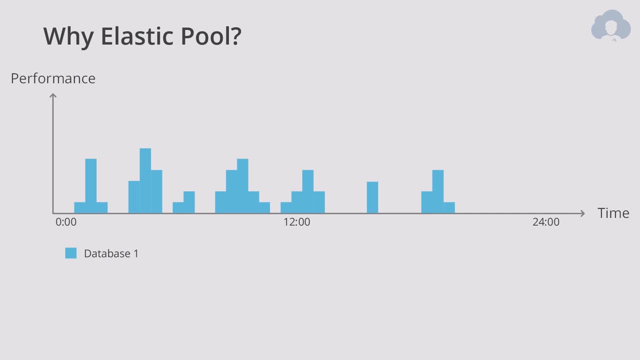 pool, since, I already said, this is a shared capacity that must involve more than one database. so if your database has very uneven use during out the day- maybe more during the early stages of the day and less during the later stages, or maybe very rarely, it's used, maybe for reporting purposes only, this will mean 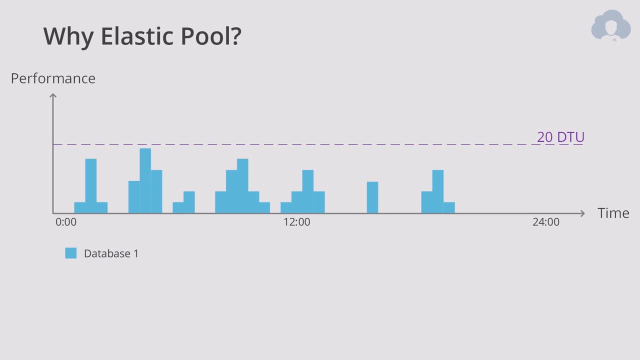 that you need to scale your database to the certain level, for instance 20 DTU, to make sure your users will never feel slow down. so a bit above what you need. but if you have two databases with similar usage but maybe differently span across the day- the second database, you will also need to scale it up to 20 DTUs. 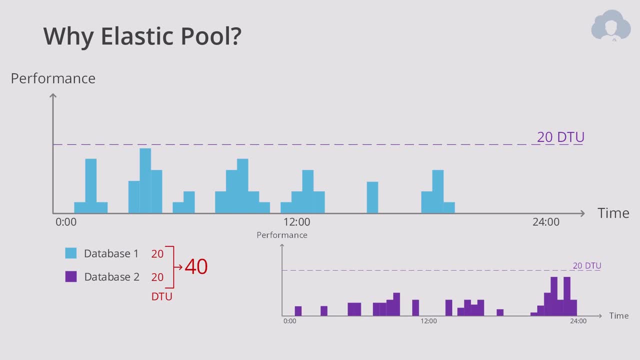 as you can imagine, that means you're paying for two databases for 40 DTUs. but what would happen if you would overlay this and put it on a single diagram? you would get something like this: as you can see, the usage spans really nicely across the day across multiple databases, even though during one period of the 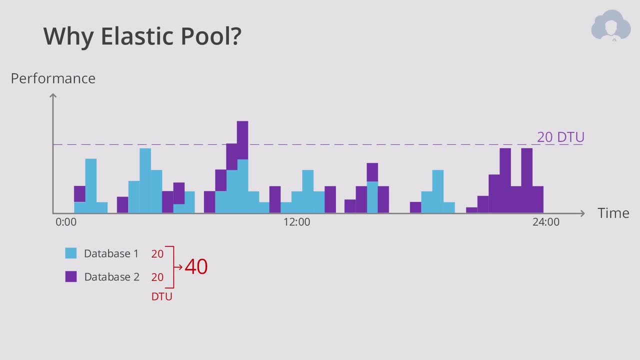 time you're overusing 20 DTUs. that means you can actually still scale to 30, but 30 DTUs is still smaller than 40, so you're only paying 30 DTUs in this case, so you're saving up money. this elastic pool allows you to share resources across multiple databases. there are 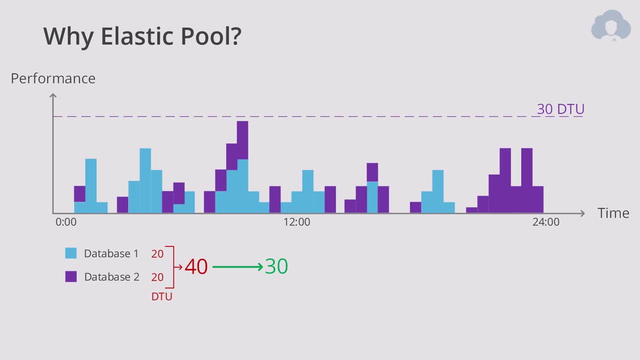 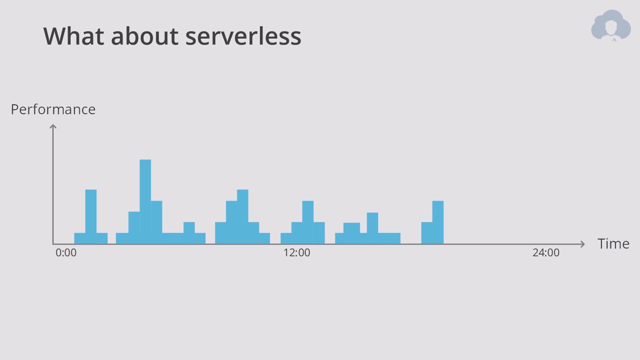 otherwise, not many databases are Hokkaidoigo, just specifically in illing to hotmail about vanda service, where u spread multiple clients into multiple databases, they willuth squared areas where your database. therefore, it's perfect for scenarios where you have many databases. what would be the center like this? well, 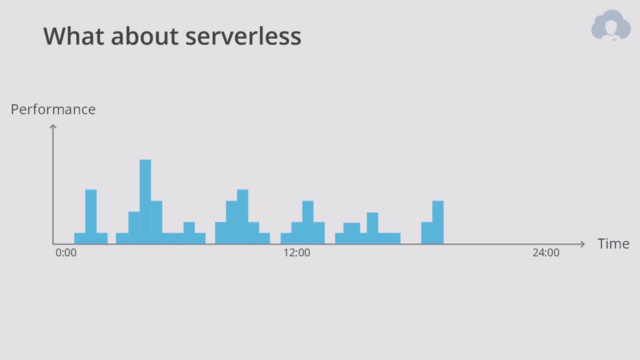 one. so you cannot share resources because you don't have to share it with anyone. but you still have very uneven usage. maybe only during the first part of the day use the database and maybe you don't during the second part. with serverless, you can actually say that you want to scale database. 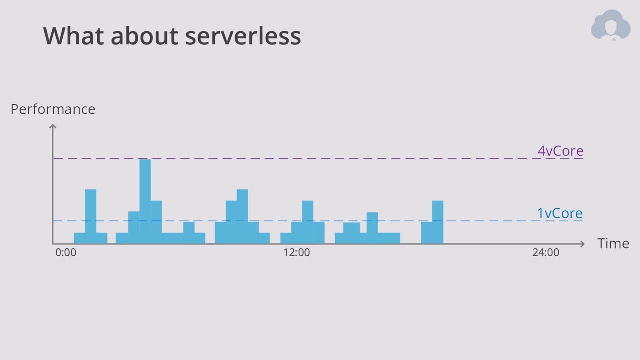 between one and four vcores, like an automatic scaling, and with this knowledge, microsoft will track your usage and, based on tracked usage, you will pay only for what you use. but notic notice something interesting: you paid only for what you use, plus a bit more. why is that? 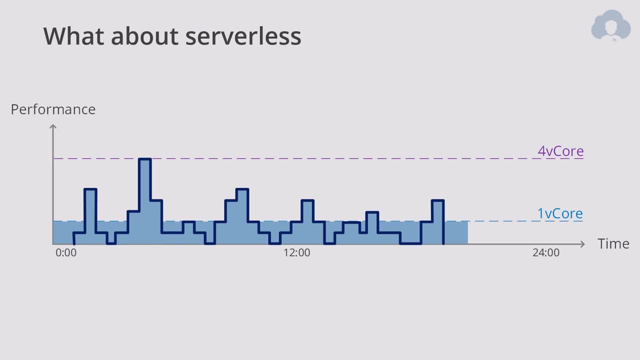 because you define that you pay minimum of one v core, so you will pay for that. but also notice something near the end here: the diagram dropped- and that's not my mistake. it was actually period of inactivity here and with serverless you can actually say that if your date 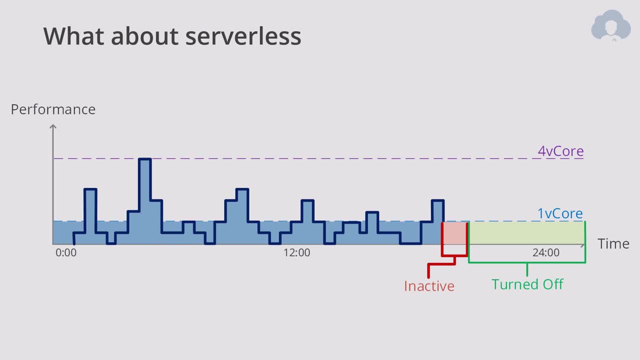 a base is inactive for some time, please turn it off, and then you're gonna pay literally zero. of course, with this model, you're gonna pay for a bit more for usage, so you really nicely need to plan your usage ahead. if you don't know, you can switch it back and forth to see what your usage is. 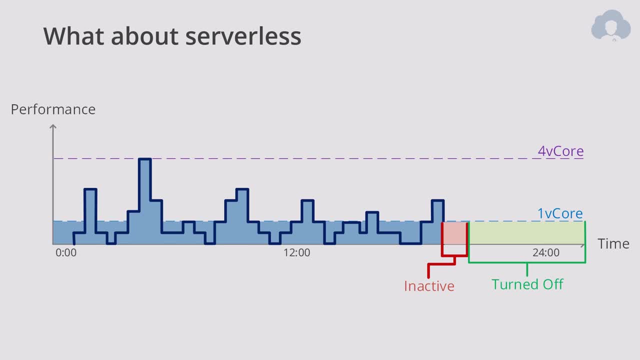 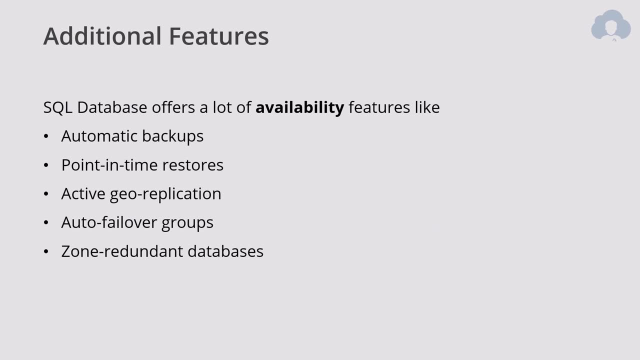 but if you do it design very nicely and you have very rare usage of database, this might be very perfect scenario for you. so that's the serverless pricing. when it comes to additional features, database is all about data quality and protection of your data, because data is currently most valuable asset on the planet. therefore, sql's database comes 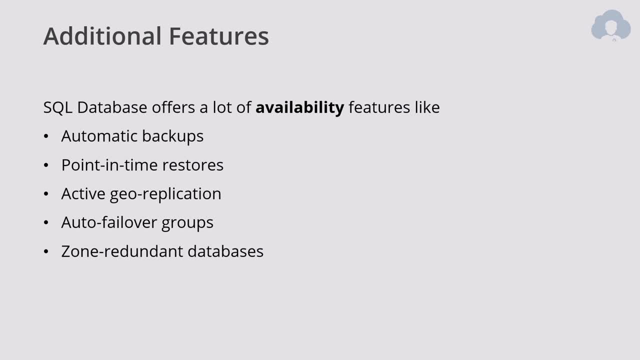 with all those availability features like automatic backups, point in time restores, so you just can one click and get back in time to specific time of your database. you have active dual replication across regions. you have failover groups and redundant databases. all those features are there for microsoft to provide you with this very highly available database and all those. 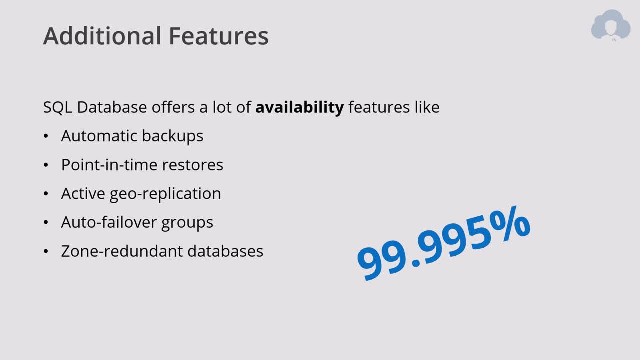 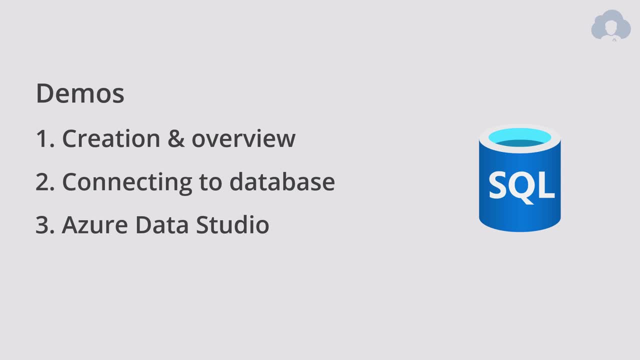 features are again for you to protect your data, store your data, manage your data and ensure quality of your data. with all that said, we can actually go to demos, and demos for today for our free creation and overview of the database. connecting to database, this time from management studio. but 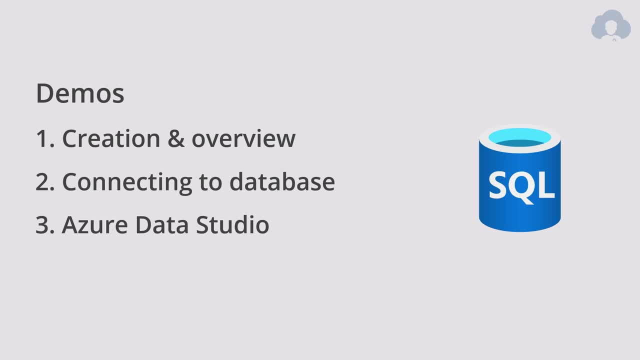 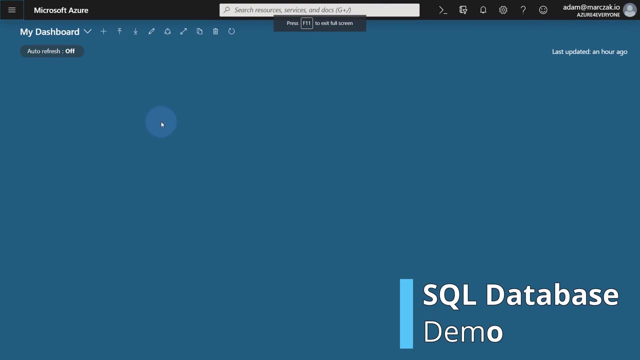 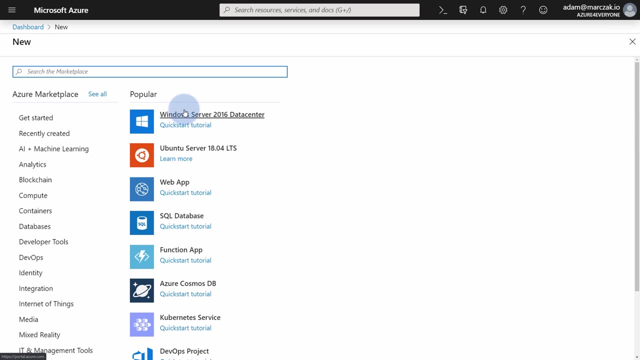 i will also show you the latest tool from microsoft, called azuredatacom- azuredatacom data studio. so let's jump right to it. so let's go into the portal. this is new look of the portal just before they ignite. so now, to create a new resource, you go here, click on the create new resource. so it's very similar. 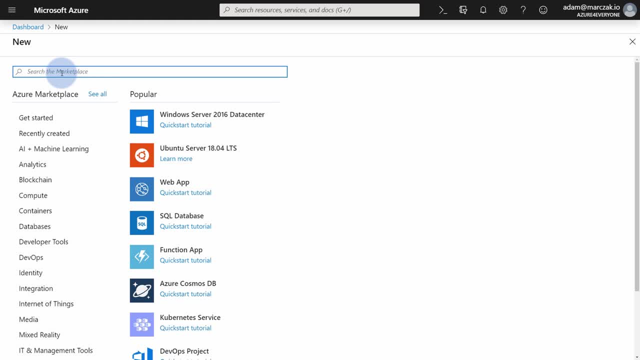 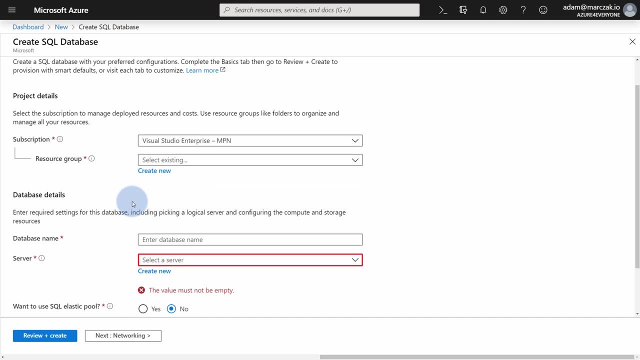 experience and you hit on sql database or just search for sql database in the marketplace. you hit create when it pops up and, of course, now you can start creating. first of all, you always need to choose resource group. you can create a new resource group or you can create a new resource group. 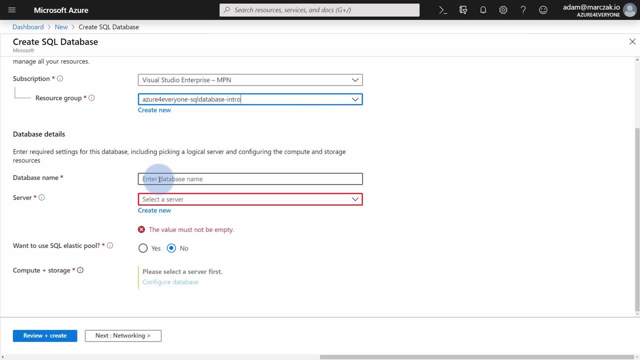 to choose resource group. when you do it, you need to provide the database name. this is again the database within the sql server date, so i'm gonna choose it. uh a for e demo db. right, and i need to choose a server. but since i don't have any server now, i also need to create server during this step. 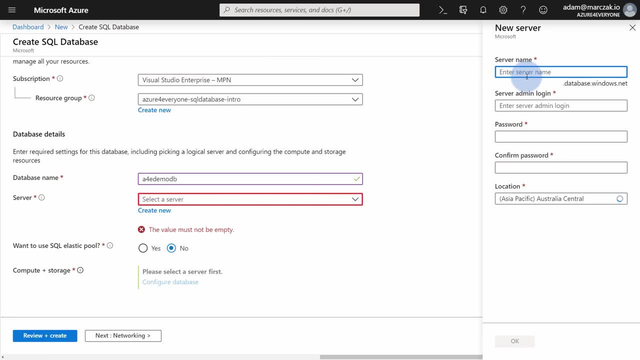 so i'm hitting on create new and i need to provide a name- a for e db server. then i need to provide an admin login- a for e admin. i need to provide a password- it's matching- and i need to provide location. as always, i'm choosing. 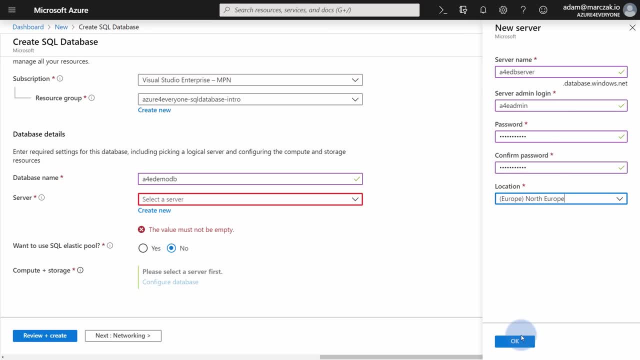 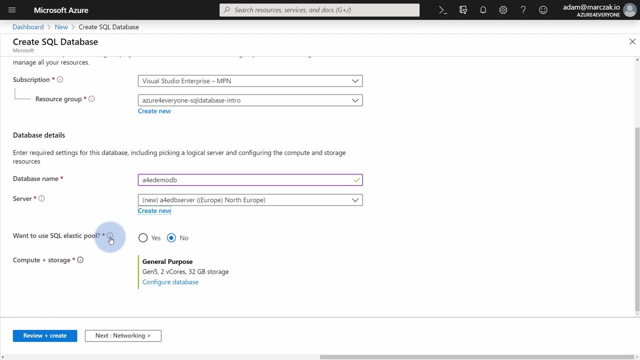 north europe because it's the closest data center to me, hitting ok and you have the checkbox: do you want to use elastic pool, as we were saying? if you have this scenario where you're going to be sharing resources, select yes. otherwise leave it at snow. and, very important, configure database because, by default, what you're purchasing will. 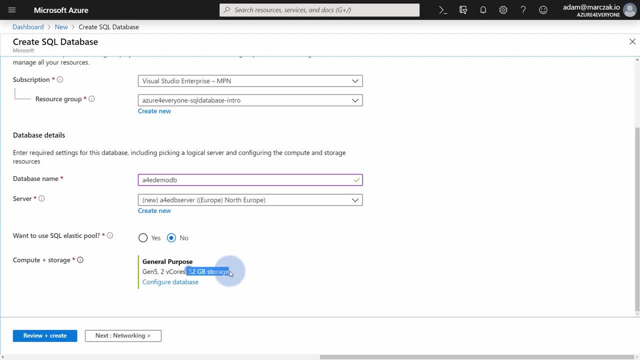 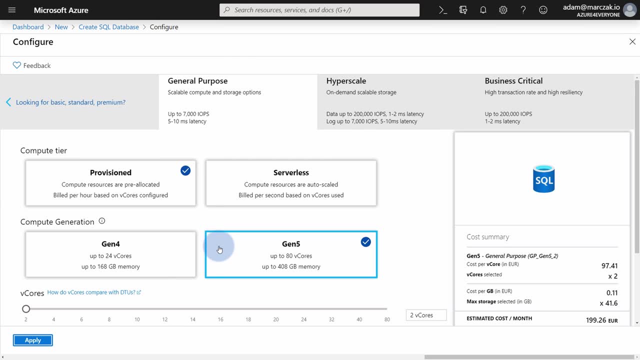 be generation 5, 2v course, 32 gigs of storage, so it's quite big database. if you're just testing, make sure to take smaller. hit on configure database and you're presented with this ui. first important thing is to notice. on the very top you have the pricing tiers, you have general. 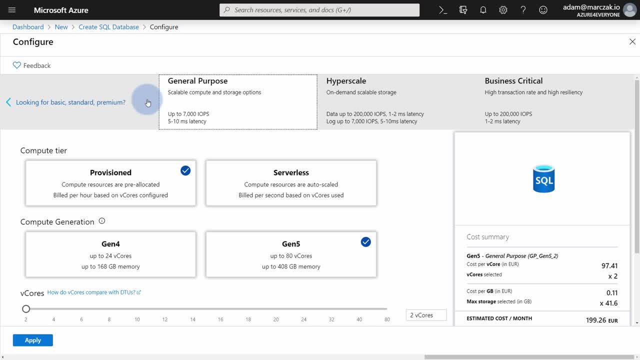 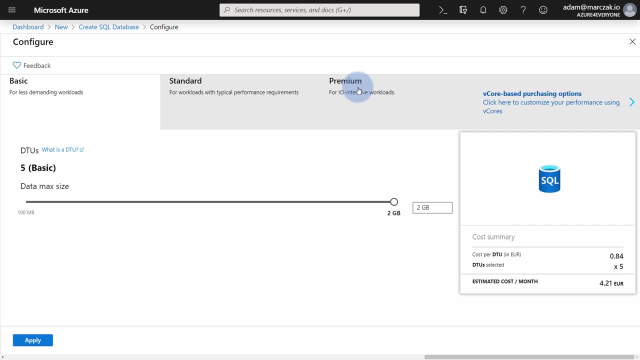 hyper scale and business critical. but also, if you look here, looking for other tiers, if you move here, you have basic standard and premium. basic standard and premium are dtu based. all of them are dtu based. notice that basic is 5 dtu. standard is from 10 to 3000 dtu. 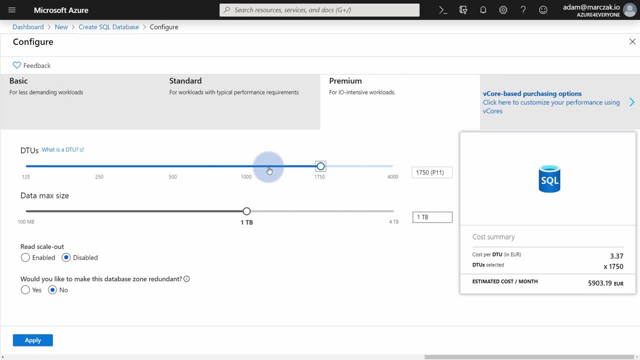 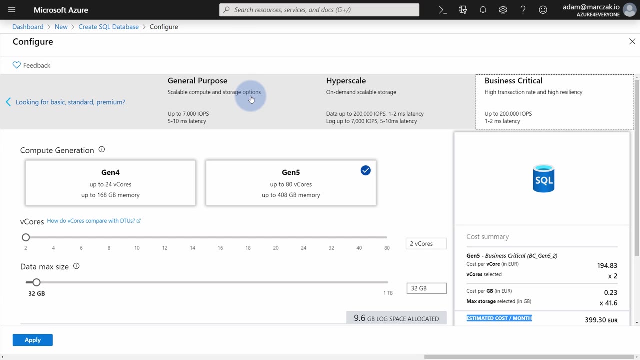 and premium is from 125 to 4000 dtu. of course, as soon as you slide that slider you get the price in estimation for your database and if you go to vcore based purchasing model, you have general purpose, hyposcale and business critical. of course, those are the more beefier type of servers as you 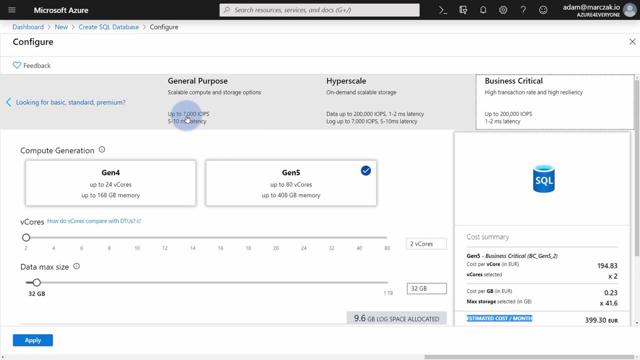 can see the most differences here with the iops right from 7, 000 iops on general purpose so operate io operations per second. so your disk speed for 200, 000 for hyperscale and business critical so getting those ssd drives really fast. drive stir, so of general purpose you can choose. how many cores do you want? 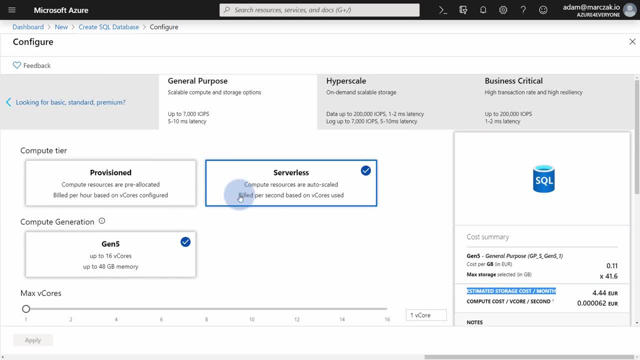 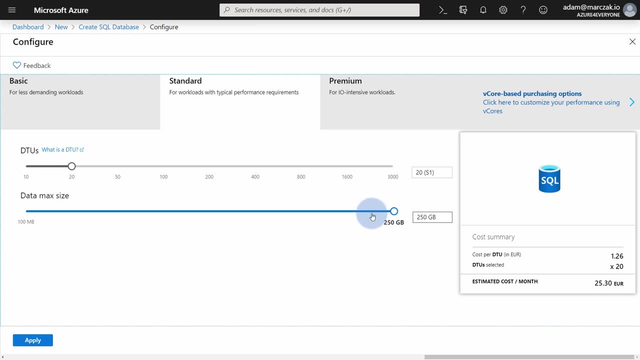 and here's also that serverless option that we're talking about. but i will actually go and create a simple database, so i'm going to choose the standard. maybe take 20 dtu and remember that we are saying for dtu, you scale storage the same way, you stay. 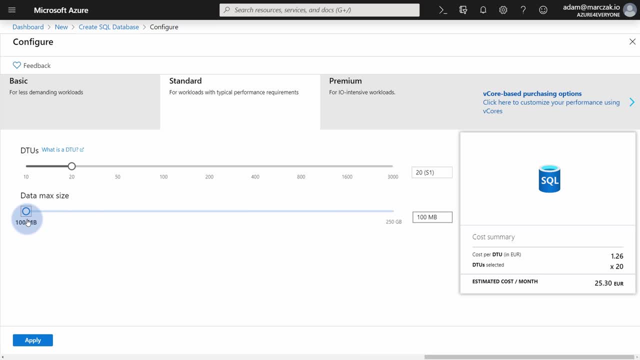 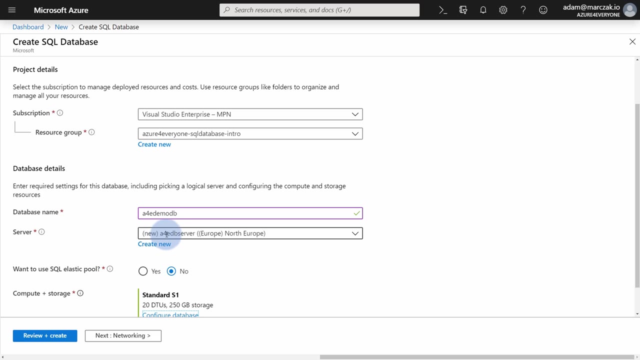 scale the dtu. so even if i move the slider to 100 megabytes, i'm still paying the same as to how many us for 250 gigabytes, because this is already paid for. so I'm just gonna leave it and hit apply. so right now we'll be creating an SQL server called a4e DB. 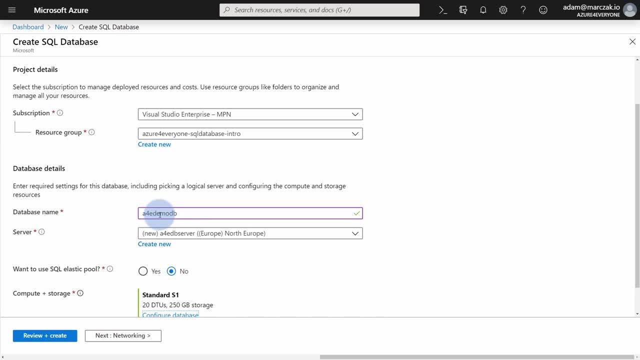 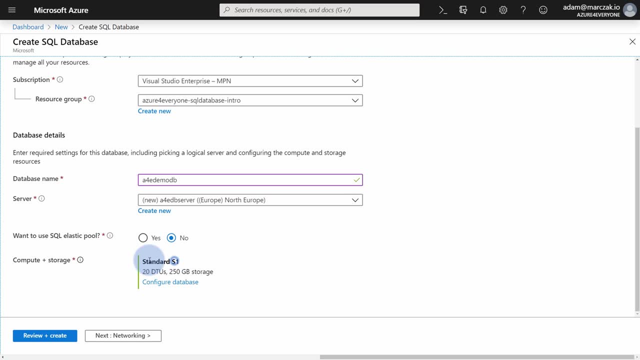 server with one database inside a4e de mod demo DB and that's gonna be pricing standard s1. so basically standard is this s and one is the position on the slider. so that's will be 20 D to use 250 gigs of storage. hit review and you can. 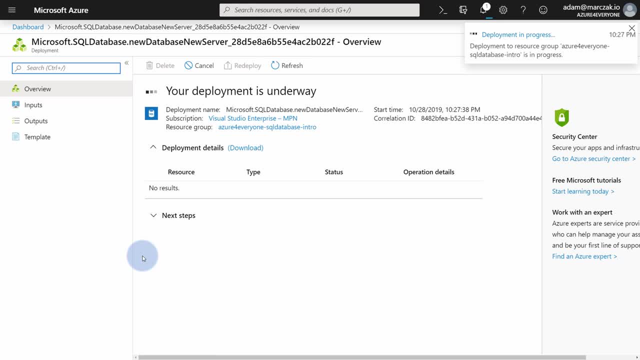 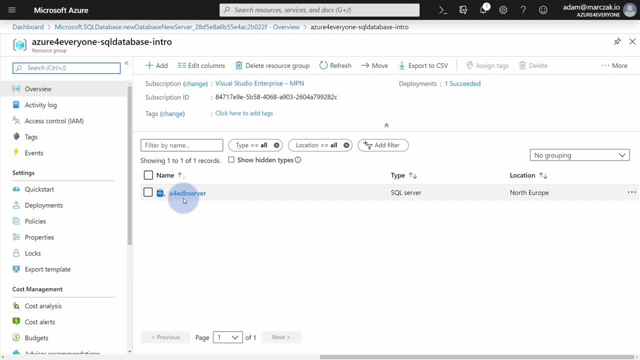 actually hit create. this will take about one minute, so I will actually skip ahead. okay, so my database was created. that means I can actually go to my resource group and see what was created. if you hit on this, it will go to resource group and you will notice that you have your SQL server here. I'll actually refresh. 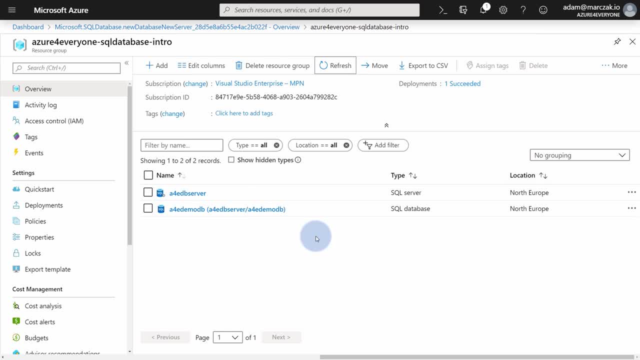 and I actually have to refresh second time to get the database. so, as we were creating, we got two resources: an SQL server- that's our centralized unit for managing databases- and an SQL database. so let's go into both to see what do we have here in the database. in the overview tab you have the most important. 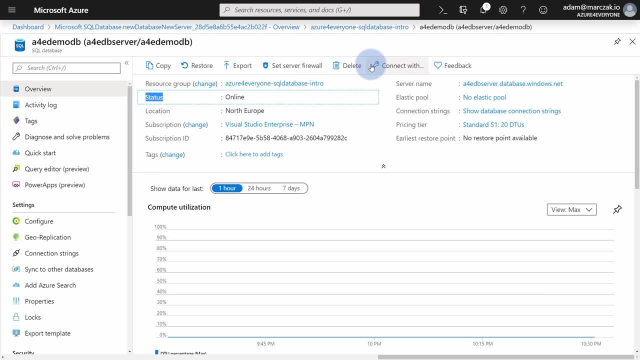 thing, the status online. notice that there is no stop button because you cannot stop database. the only tier that allows you to stop database is the server last. otherwise you will pay for entire month of usage, regardless if you use it or not. the only thing you can do to reduce costs is scale pricing tier. you have the 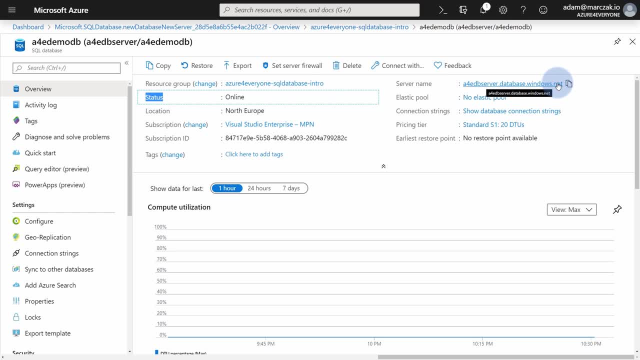 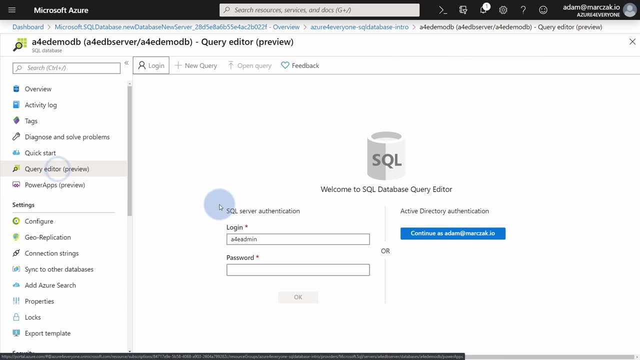 location. here you have your server name. this is the server that you will use for the connection string to connect to database. there are no currently elastic pulls assigned. you have the pricing tier here and on the left hand side you have couple cool features. the query editor allows you to connect to the database. 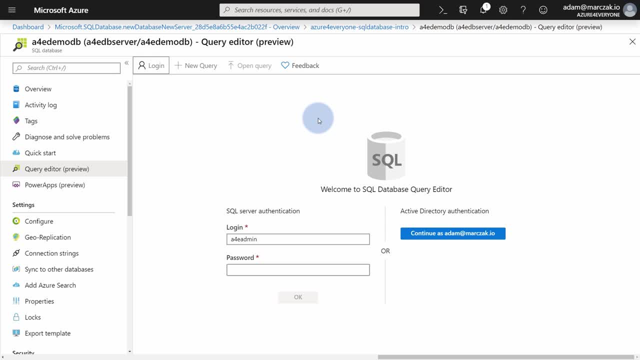 from the browser and manage your database. I don't really recommend this because this requires you to open public IPs to be able to connect from the browser, so let's leave that for now. especially, this is in preview, so you might not know when this will be taken. 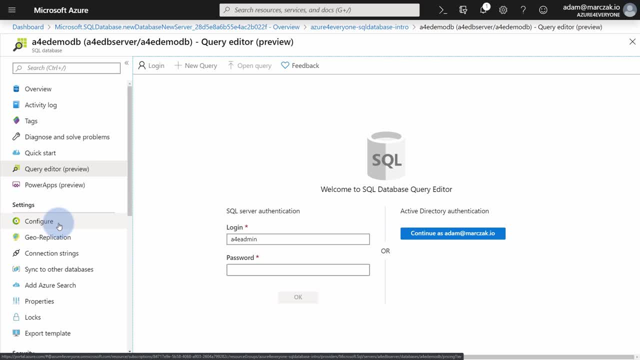 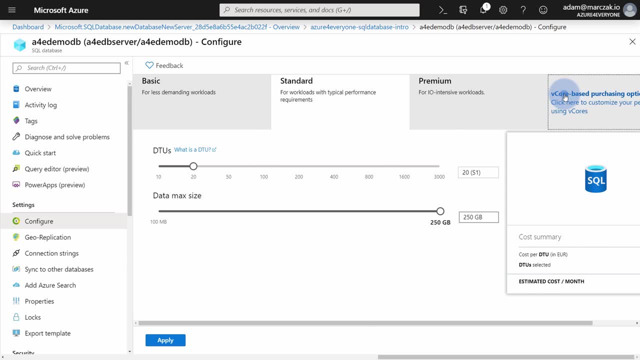 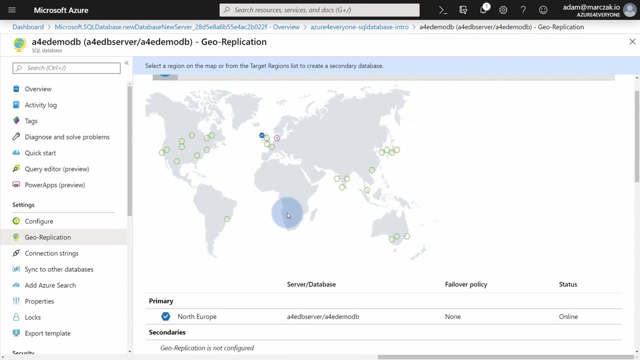 out or maybe productionized. so what do we need? first of all, configure so even after creation of database, you are always allowed to change that reader back to any V core or DTU based tiers. you can go to Jira application and if you want to add some read replicas, you can do it here and just select which. 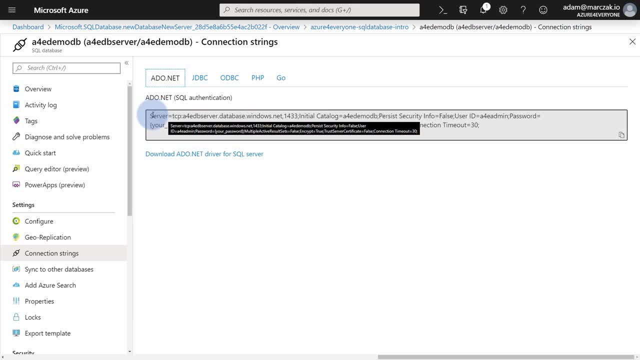 region, do you want it? you have connection string tab so you can just copy your connection string. this tab is pretty cool because you have a do net. you have JDBC if you're working with Java, ODBC by PHP or go even sample code to connect to this database, so it's pretty neat. you have also sync, so you 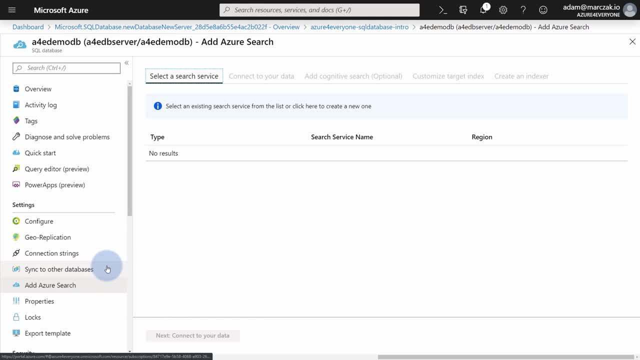 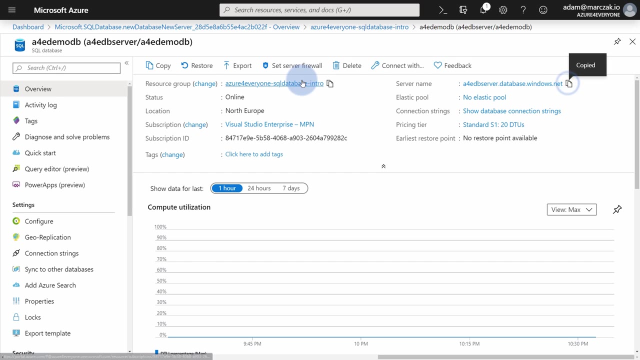 can actually sync to other databases. you can add Azure search, so integrate with many services. you have advanced data production and some other stuff about security, but what we need so far? now let's do something simple: let's connect to this database. so I'm gonna grab the server name and on the second screen I'm 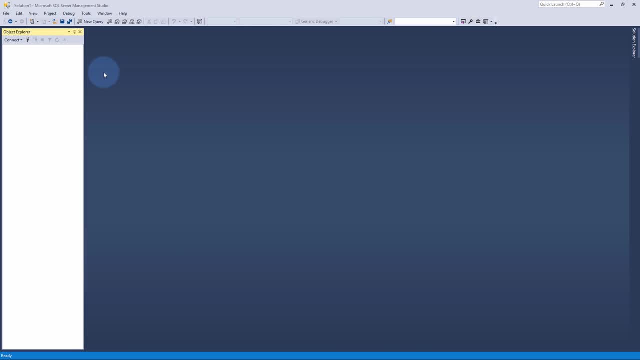 gonna use SQL Server Management Studio, this free tool, and most of the people in the market knows this tool if they've been working with SQL Server. to connect, you need to hit on connect, hit database engine, paste in the server name. you need to paste in the server name. you need to paste in the server name. you need to. 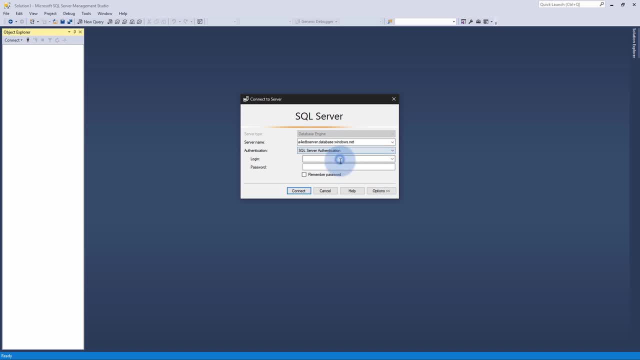 paste the name and you have two options here. you either use SQL Server authentication. this is the account that you set up when creating. in our case, this was a for a admin, but you should actually never use this. you should always use Active Directory Universal, so your actual Active Directory account to. 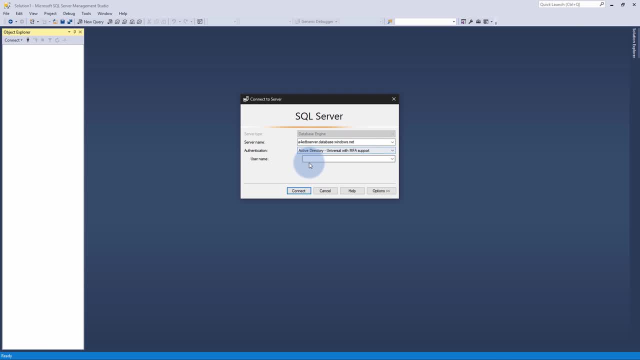 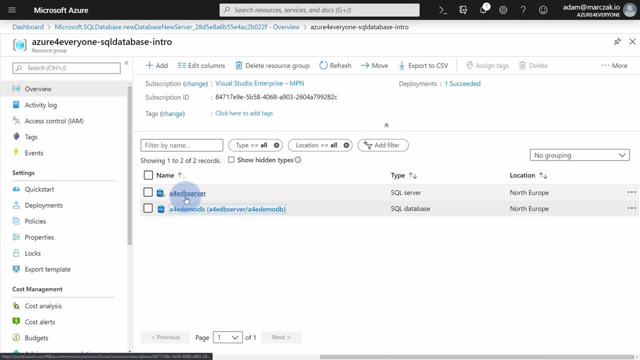 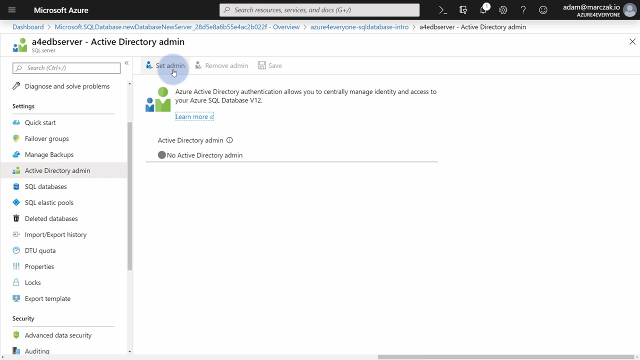 be able to log into this server using this Active Directory. you need to first set yourself as an admin to do so. you go back to database here, go to the server and on the server you will have the section here: Active Directory admin. what you just need to do is set. 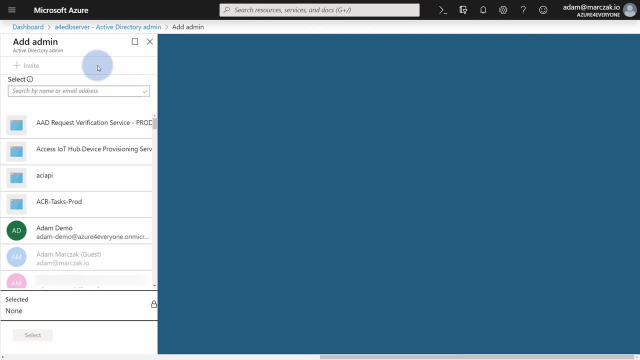 admin. so now you can actually set admin. but notice, interestingly, I cannot use my own account. this is because my account is a guest account in this Active Directory, so I need to use account from this Active Directory, like the one that I set up before. so, Adam, demo at Azure for everyone calm. so you just hit on it. hit. 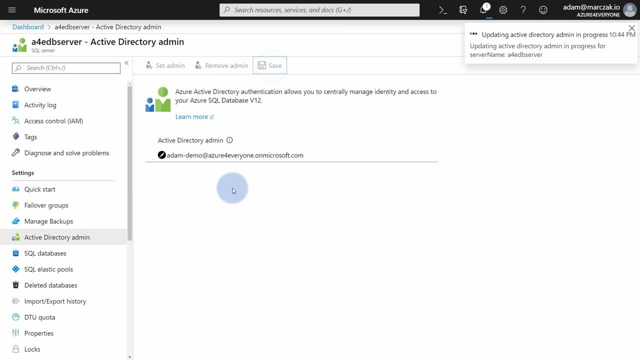 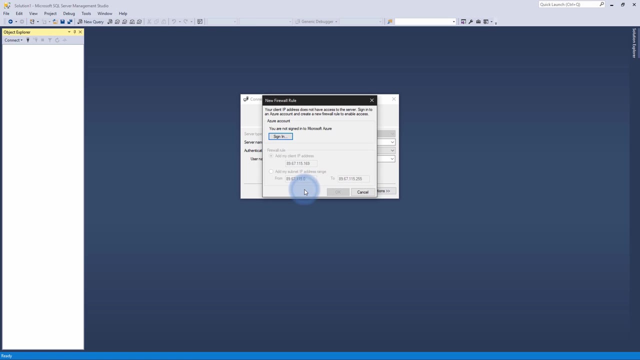 like and remember to hit save. now I can actually login as an administrator to this SQL Server using my Active Directory account that they created previously, so I just copy paste this name, go back to SQL server, paste it, hit connect and notice. interestingly, I got a pop up that SQL. 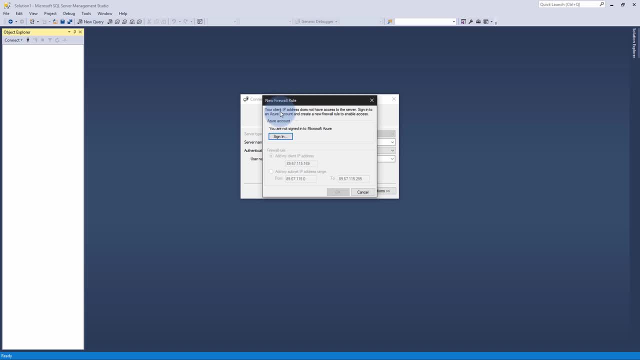 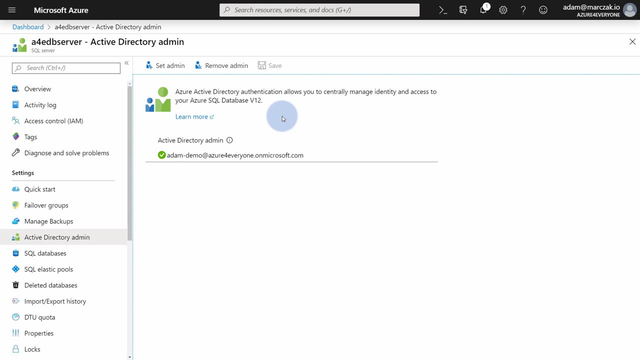 Server Management studio recognized that there is no firewall rule allowing me to connect, so currently firewall is blocking me to connect to the server server, and this makes sense because SQL, as we said, is all about protecting your data, so it does not allow anyone accessing by default. so what you need to? 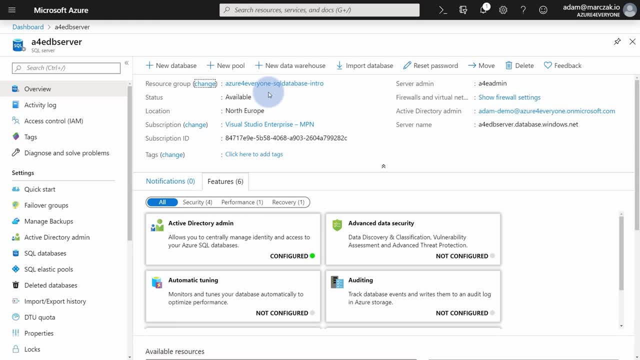 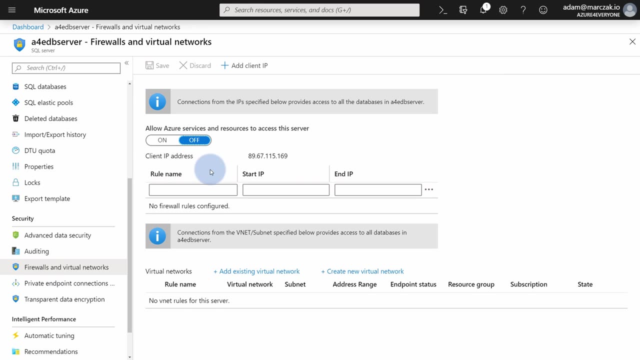 do right now is go to overview and you need to go to server because, we already said, the firewall is managed on a server level. so you can actually find the server level firewall settings here, firewalls and virtual networks. in here you have the client IP address. that's my current IP, my current public IP, which I 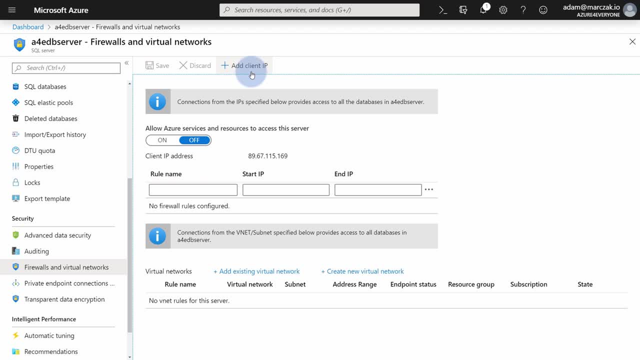 need to add in order to be able to connect to database. to do so, I cannot just click this add client IP, which will add additional row in this table and I can just call it Adam home. this way, I will know that this IP is my home IP. 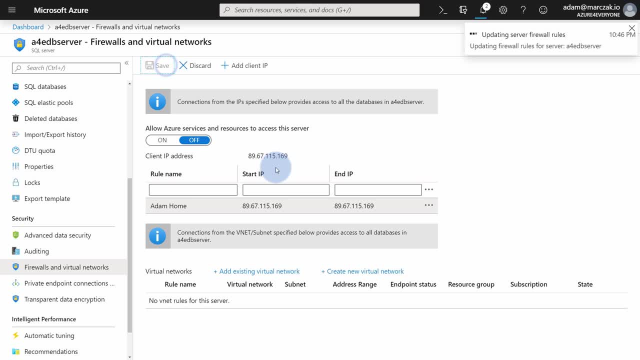 that I will be connecting from and I just can hit save, since my IP is dynamic. I might need to come back here in future and change it, But for now this should be okay. So if I go back here and actually cancel this and hit connect again, 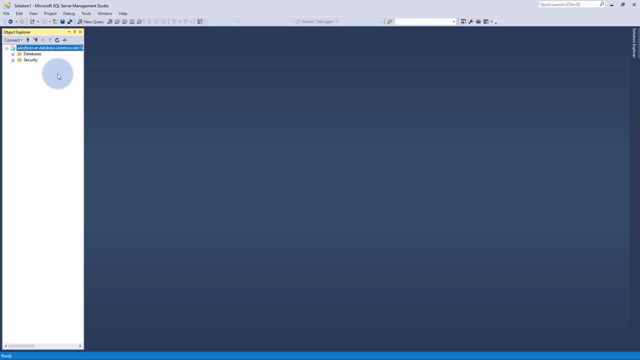 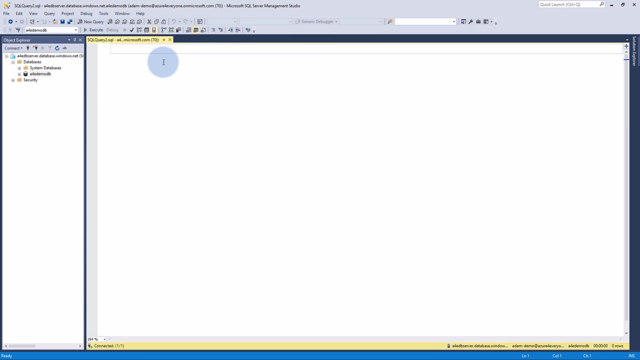 Right now I Connected the reason they didn't ask me for credentials because I was already connecting using this account previously, So it remembered my credentials. but of course if I open my database I see my a4e demo DB And then again just click new query and start querying my database. 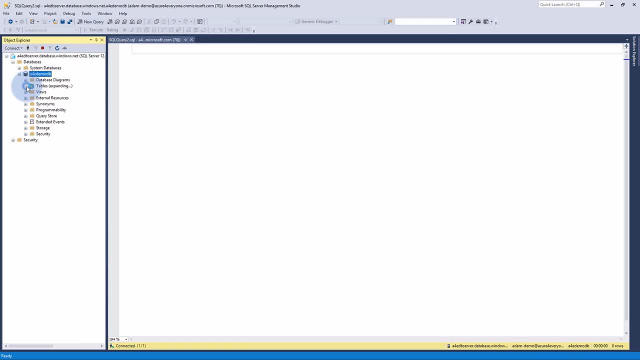 Of course, within that database, out of the box, There are no tables, No views, No nothing. So what we can do right now is actually create some views and maybe create a table. Okay, so let's create that person's table that we were using during the demo. 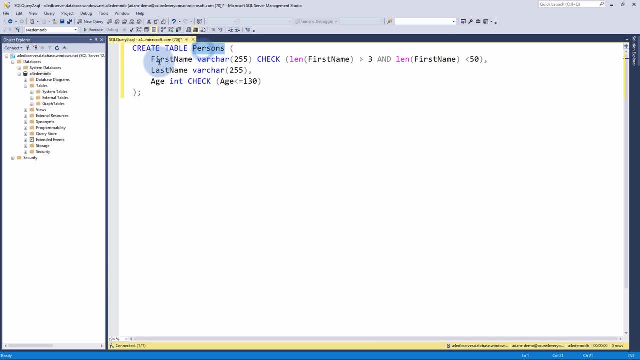 So it would be: create table statement- persons, three columns and some constraints. just gonna run it command Completed successfully, you can refresh table And see your table being there. if you can expand it, see what are the columns, what are the constraints, Everything that just created, and if you want to add an additional row to this table. 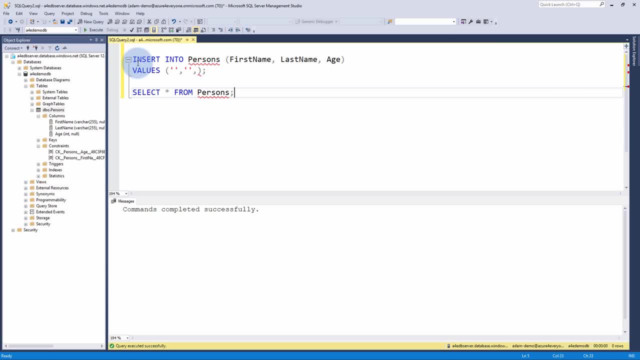 You can simply Add a query, insert into persons first name, last name and age and then put some values. if I would type a Marchak 32, this will actually fail, because if I run that This now, it will conflict with the constraint that we said, because the name has to be longer than three letters. 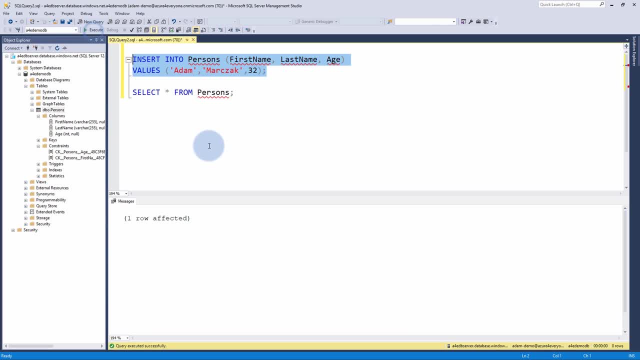 So if I'm gonna type Adam and just run it, it runs successfully. you can now just select from the table to see our data there. This is as simple as it gets, because database is about putting data there. Think, figure out your database model for your business needs and just using it. 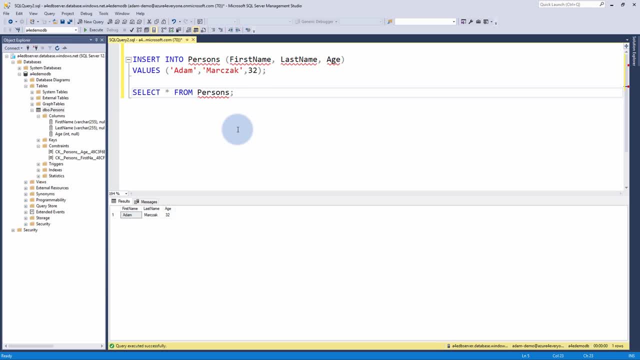 So the very last demo that we want to do is pretty much similar to this. Let's open the same scenario using Azure Data Studio. Azure Data Studio is the newest tool from Microsoft, allowing you to also connect and work with Azure SQL database. so this looks like like that, and if you been working with SQL and 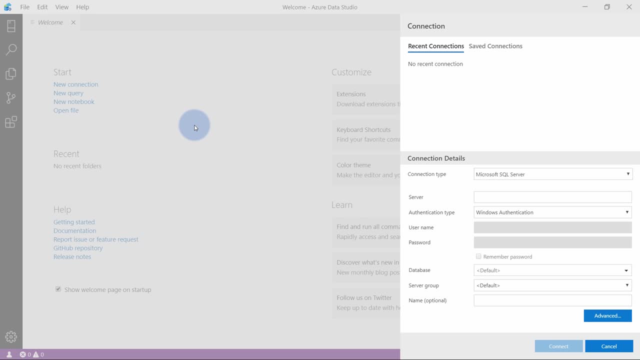 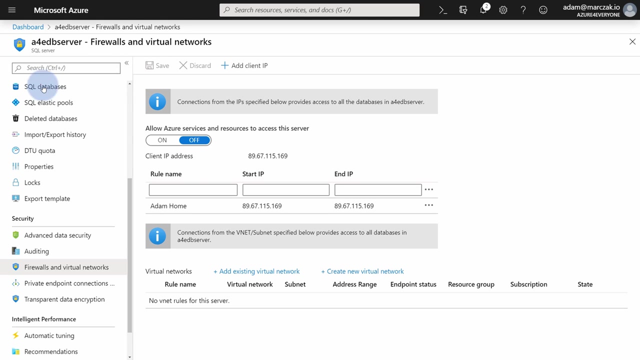 You've been working with Visual Studio code, You might recognize this is very similar UI. So what do you need to do here? You need to select connection type: SQL Server. you need to provide server name. so let's actually grab this from our portal. So I'll go actually go back to portal. 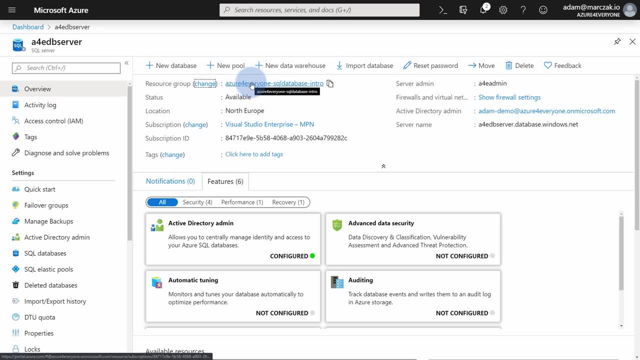 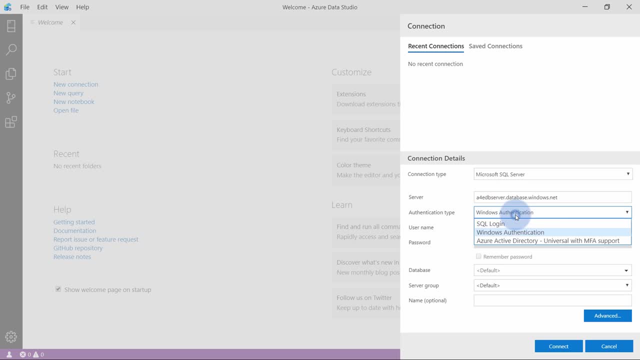 Go to overview, Go to there. actually, here's the server name, So let's copy that. Let's go to connection here. and, Of course, we're not using a SQL Server login. We're using Active Directory login, so we need to add an account. 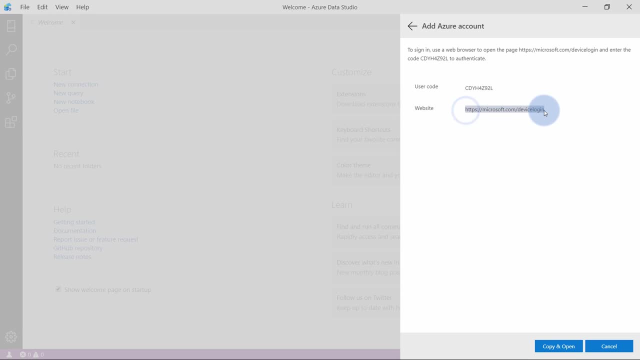 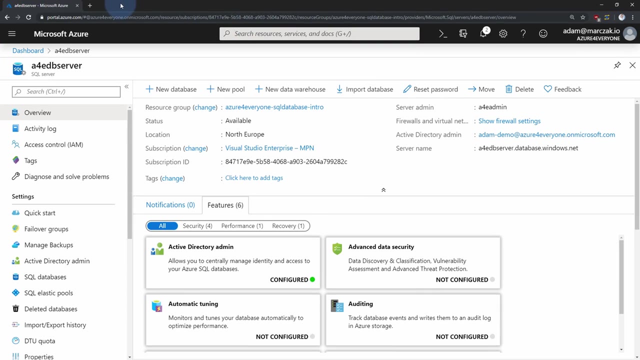 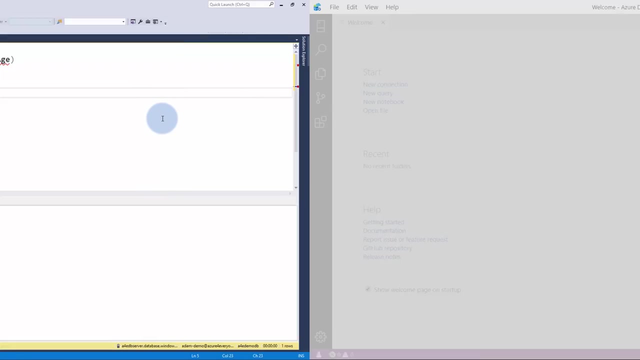 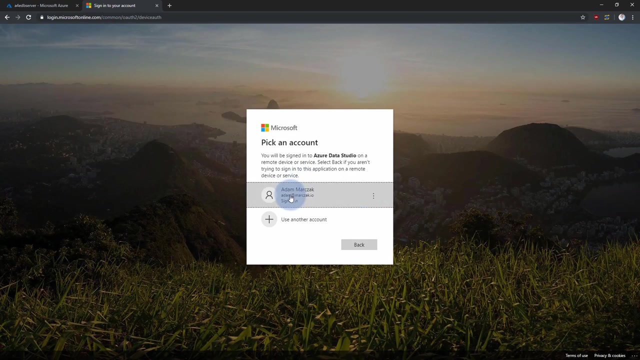 When you add an account, you will get this pop-up. You need to go to this website. So let's go to this website. F11- Open this website. It asks you to provide a code. so you need to provide this code and Login. and Now it asks you: do you want to use the account that you're currently signed in? if I will be using this to connect, 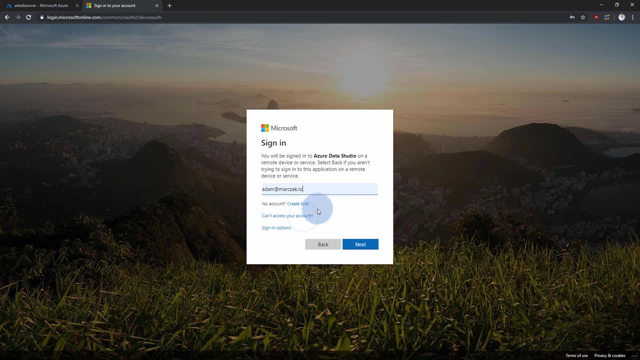 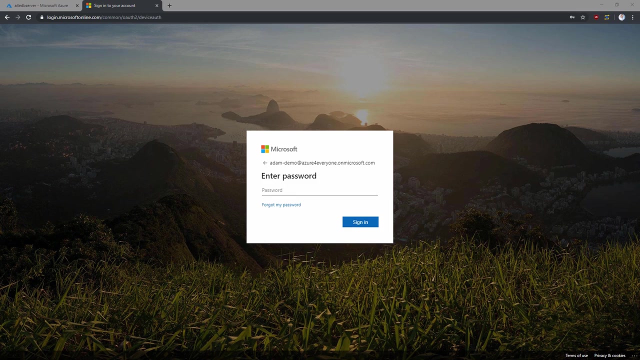 I could do so, but I need that account That I specified as an admin, so I'm gonna remove this and copy my account, so, So let's paste that in. That was our Adam demo account. go next, provide a password And just copy the password and it says: you have signed into our data studio. 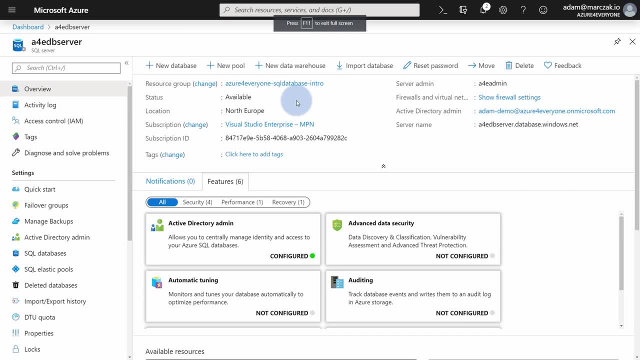 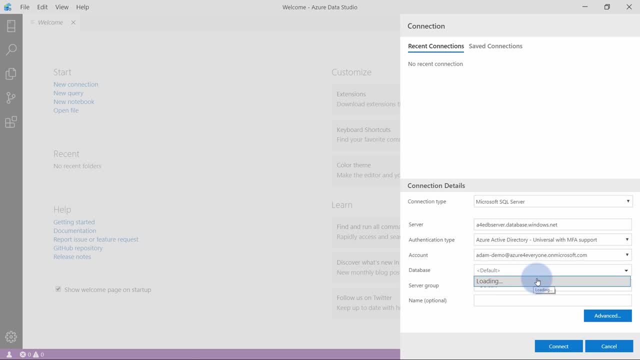 You can actually close this tab at that point- full screen that- and go back to the data studio. Notice that I'm ready logged in. If this works, I can actually expand database section to get the list of databases, because I've got master and a for a demo DB. 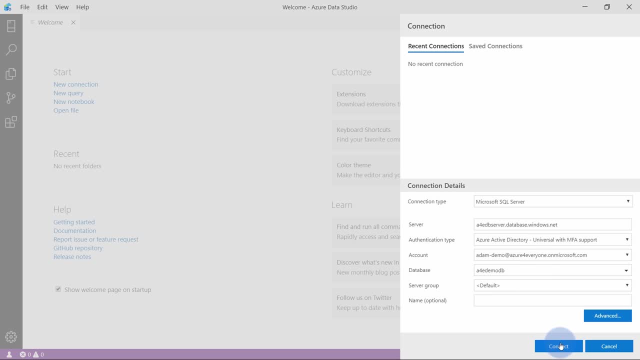 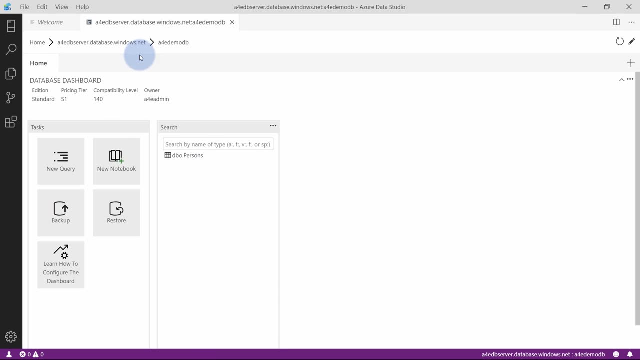 That means I logged successfully using this account, I can actually hit connect and Right now I'm in the database, the same way I did using data studio. The interface is quite different, but I like this interface much more than the visual studio. I started on the management studio because it has new features. 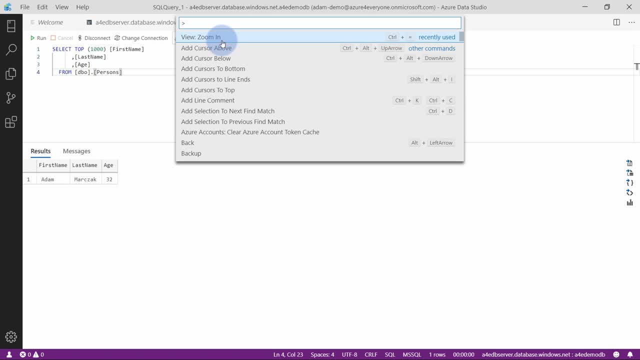 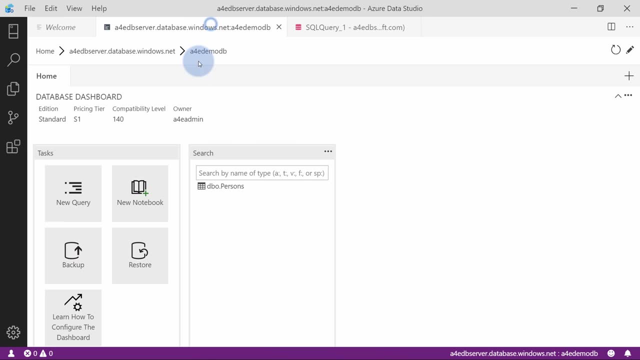 it scales nicely with UI because you just simply simply hit f1, go zoom in. an entire interface zooms in and There's new features coming in, because you have some notebooks, queries, backups, restoring- an additional feature coming in. You have even get integration from here, but this tool is very similar, as you see. you can just select from your table and 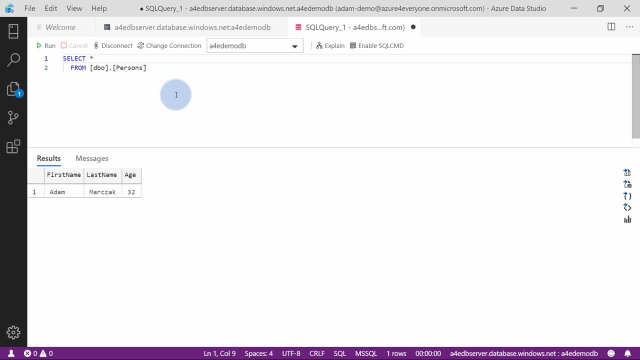 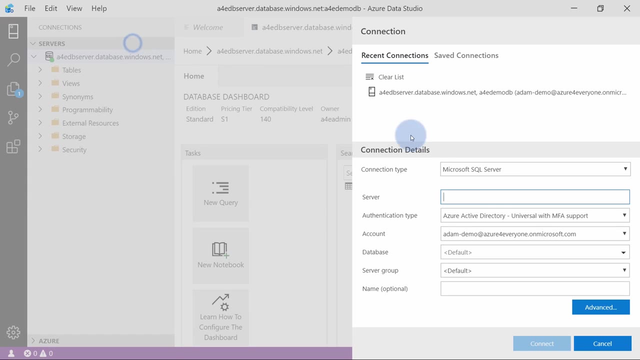 Just run it. Same stuff with management studio. same stuff here. This tool is just more simpler. But one of the cool feature is that first of all, it remembers connections So you can actually save those connections for later use and if you're connecting to more databases, When you're adding more servers, you are also already logged in. 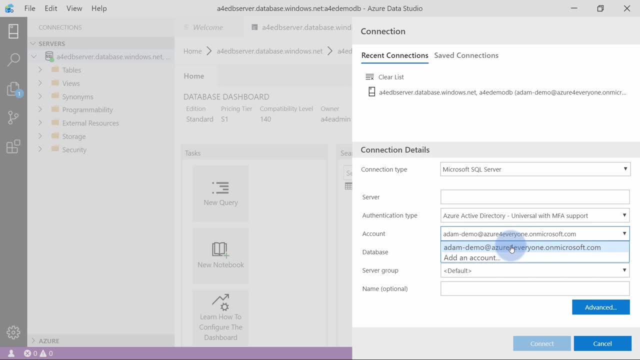 That means if you're using same account across multiple databases, you will only have to log in once to connect to all of them. There's a lot of good features here, So I really advise you to use data studio. So if we go back to the portal, what else do we have here? 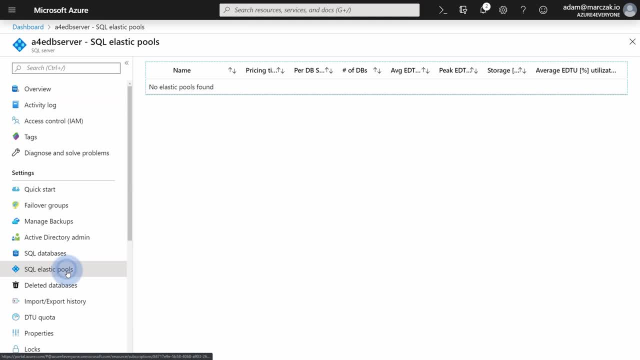 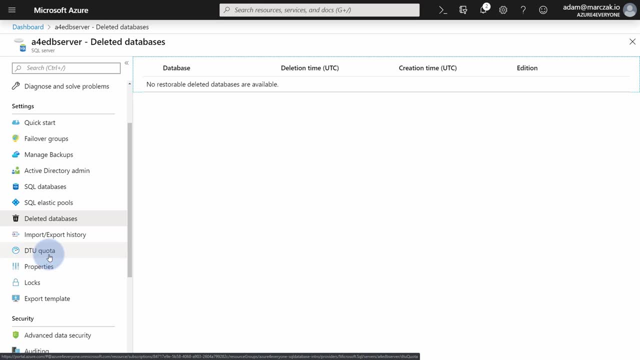 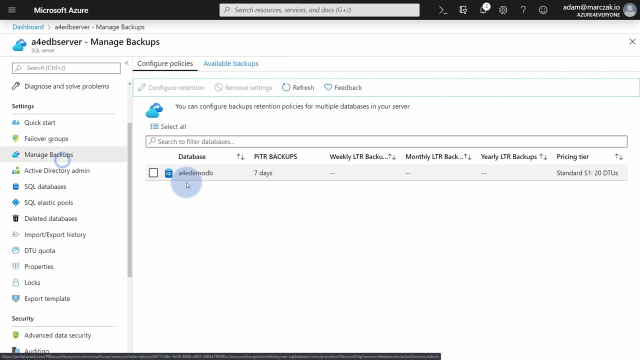 Of course, on the server level you have a bit more options. You have SQL Elastic pools here, if you want to, you can see your deleted databases. if you delete some, you can Track your quotas here. You can import and export database a lot of stuff. You can manage backups here. 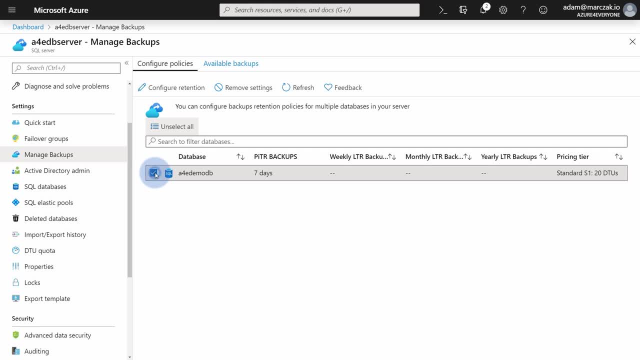 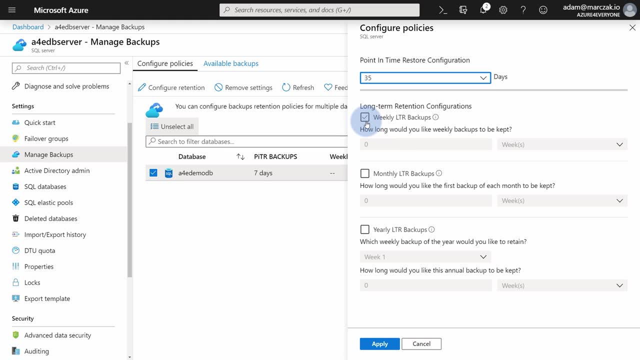 So by default your database is only backed up seven days. You just click here, configure retention And change it to any value you want, for instance 35. or maybe you want to do some long-term retention and type 365 for entire way, Year of backups or simply just one. 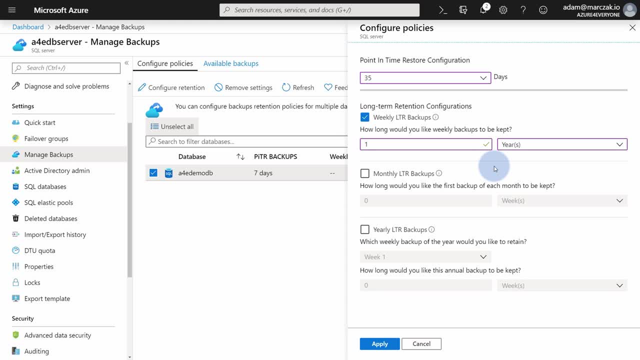 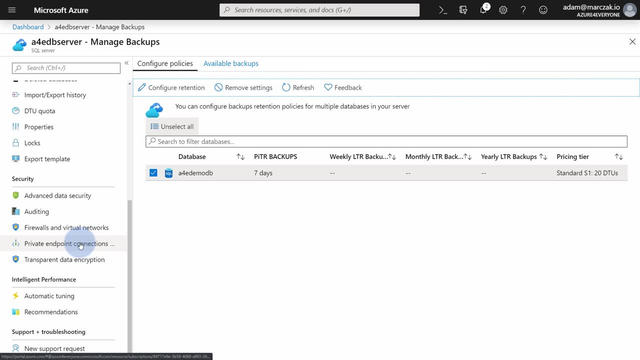 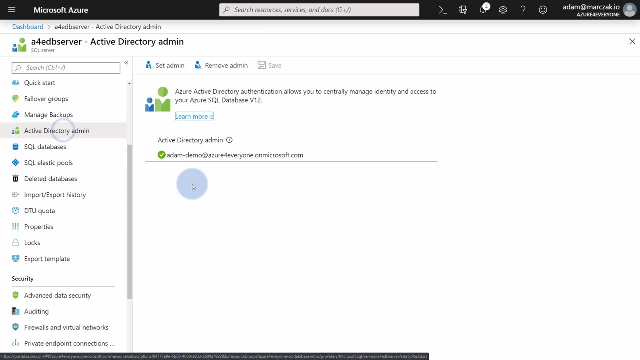 year, right. So this is how long your backups will be configured, and it's just few presses of a button: hit, apply and it's done. There's quite more features here, But to summarize the most Important one: always set yourselves as an admin to database so you can connect using your account. 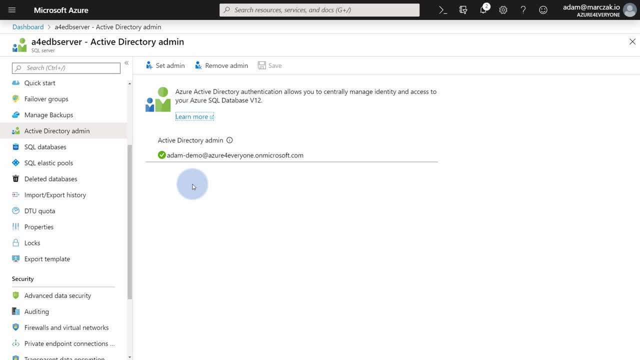 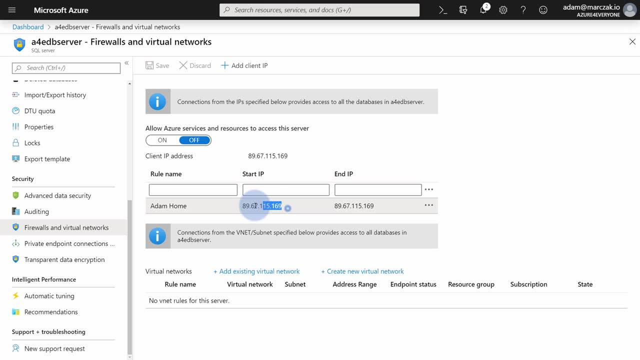 Literally, you can actually forget about that. Active Directory admin account should really never use it anyway. Remember about firewall rules, because by default, it will not allow you to connect. this goes for all the public Services as well. if you're using data factory logic apps, your web application,